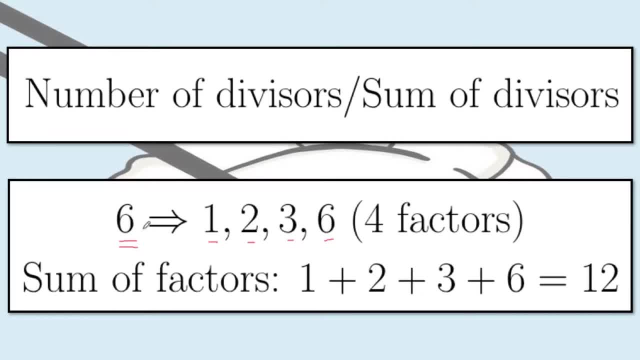 3, and divisible by 6.. Now there are no other positive integers other than these. 4, that 6 is divisible by Now. the sum of divisors very simple: just simply add all the factors, So 1 plus 2 plus 3 plus 6, and this gives us 12.. 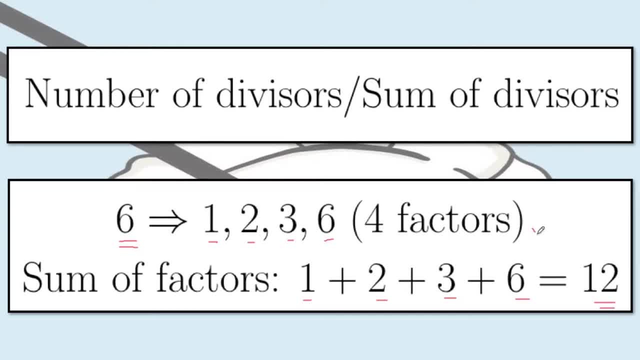 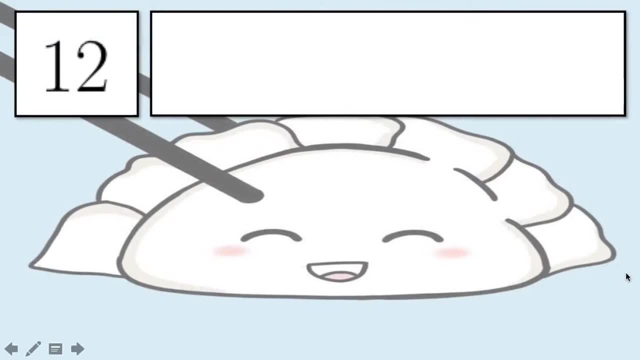 This will be telling you guys a shortcut or a method for you to get the number of divisors and the sum of the divisors of a positive integer easily. So let's start with the first positive integer, Let's try to deal with the number 12.. We can. 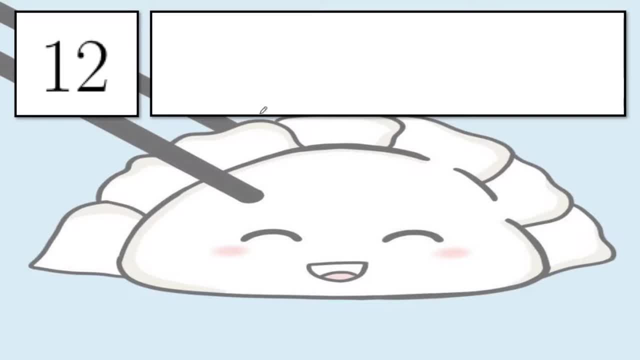 always write the positive integers, sorry, the positive divisors of 12.. So I write 1 plus 3 plus 4 plus 6 plus 12.. Since 12 is divisible by 1,, by 2,, by 3,, by 4,, by 6, and 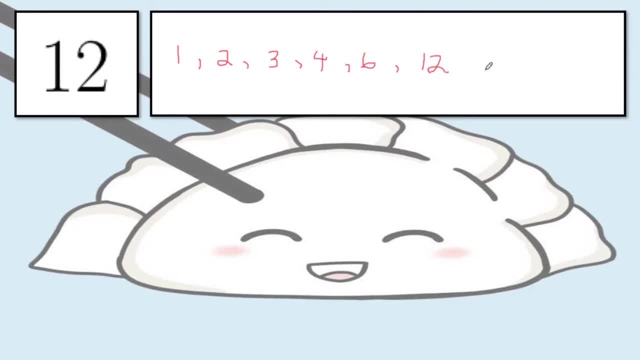 then by 12.. Now, listing them all down, there are a total of 6 divisors, so there are 6 factors of 12. And if I add all of them- 1 plus 2 plus 3 plus 4 plus 6 plus 12, I should: 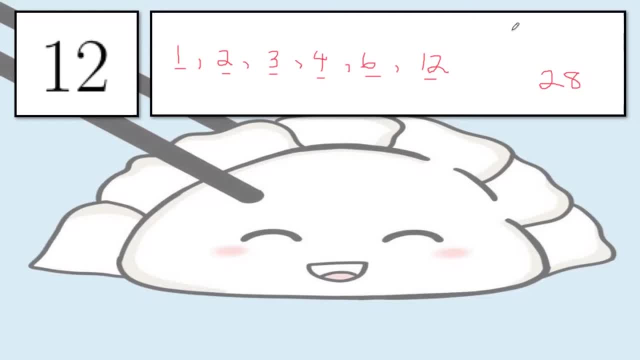 be getting 28.. The sum of the divisors is 6,. the sum of the divisors is 28, and this is indeed correct. Now, how do we get this? using a shortcut. So the first key step is for you to be able to. 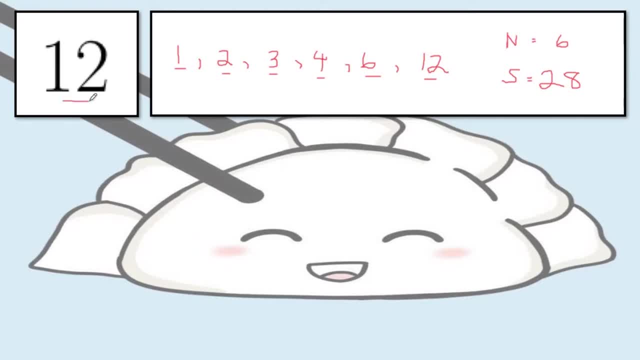 prime factorize the number. So we want to be able to prime factorize 12.. Now recall our prime factorization and we can write 12 as a product of prime factors. So 12 here has a prime factorization of 2.. 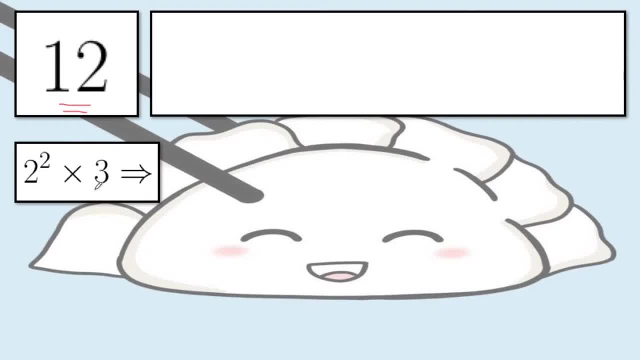 2 squared times 3.. Now we need to prepare two expressions for us to be able to get the number of factors and the sum of the factors, or the number of divisors and the sum of the divisors of 12.. Now for the number of divisors. we need to check the exponents of each prime. 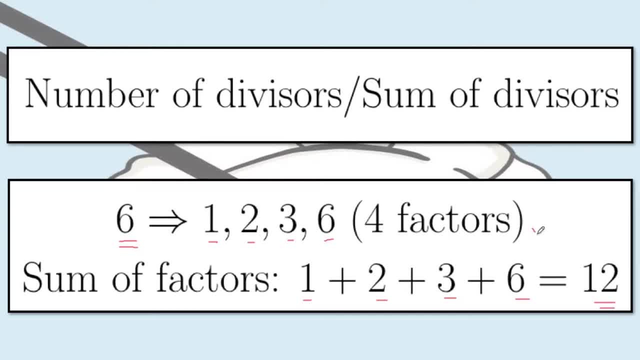 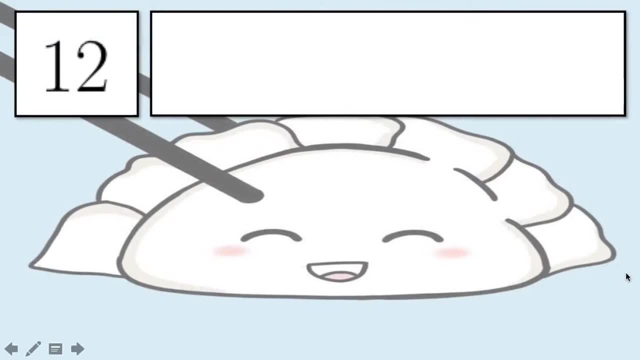 This will be telling you guys a shortcut or a method for you to get the number of divisors and the sum of the divisors of a positive integer easily. So let's start with the first positive integer, Let's try to deal with the number 12.. We can. 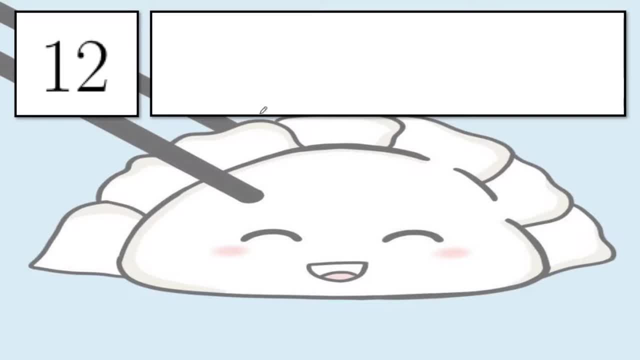 always write the positive integers, sorry, the positive divisors of 12.. So I write 1 plus 3 plus 4 plus 6 plus 12.. Since 12 is divisible by 1,, by 2,, by 3,, by 4,, by 6, and 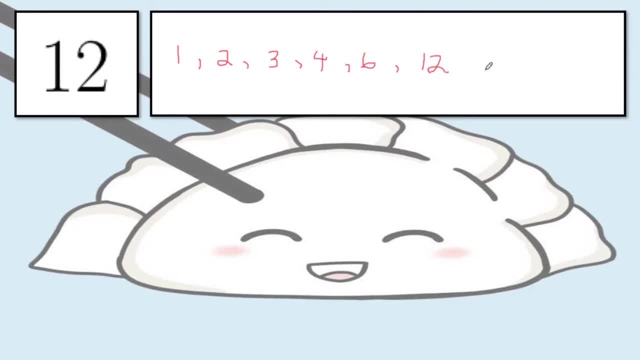 then by 12.. Now, listing them all down, there are a total of 6 divisors, so there are 6 factors of 12. And if I add all of them- 1 plus 2 plus 3 plus 4 plus 6 plus 12, I should: 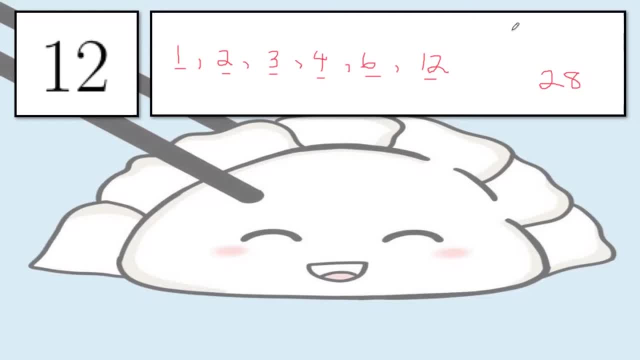 be getting 28.. The sum of the divisors is 6,. the sum of the divisors is 28, and this is indeed correct. Now, how do we get this? using a shortcut. So the first key step is for you to be able to. 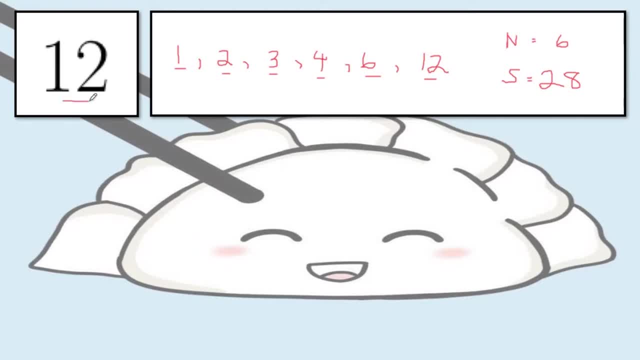 prime factorize the number. So we want to be able to prime factorize 12.. Now recall our prime factorization and we can write 12 as a product of prime factors. So 12 here has a prime factorization of 2.. 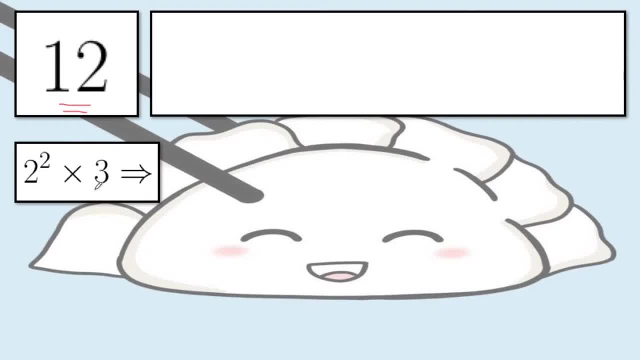 2 squared times 3.. Now we need to prepare two expressions for us to be able to get the number of factors and the sum of the factors, or the number of divisors and the sum of the divisors of 12.. Now for the number of divisors. we need to check the exponents of each prime. 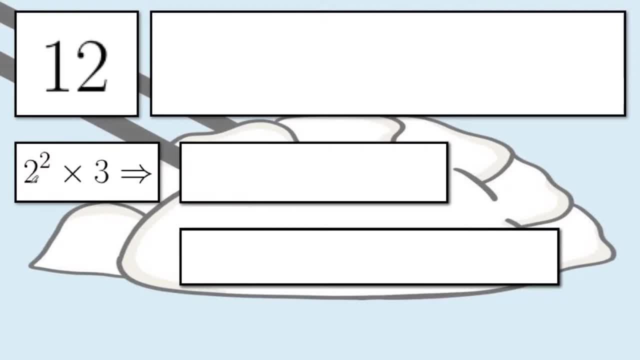 number in the prime factorization. So the power of 2 here is 2, and the power of 3 is actually 1.. So 3 raised to 1.. Now the next thing we have to do is we add 1 to all of the exponents. Now, since there 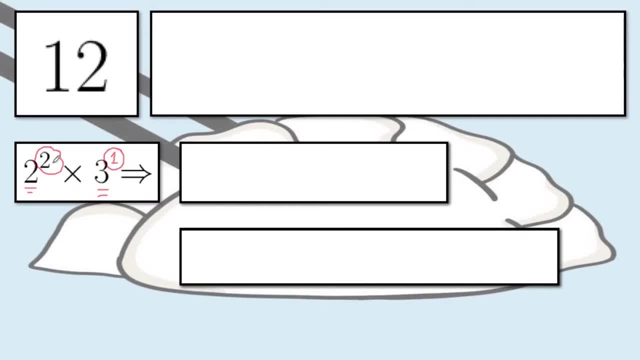 are two exponents, we will have two numbers that we multiply together, So it's not 2 and 1.. We add 1 to both of them, so it's going to become 2 plus 1 times 1 plus 1.. 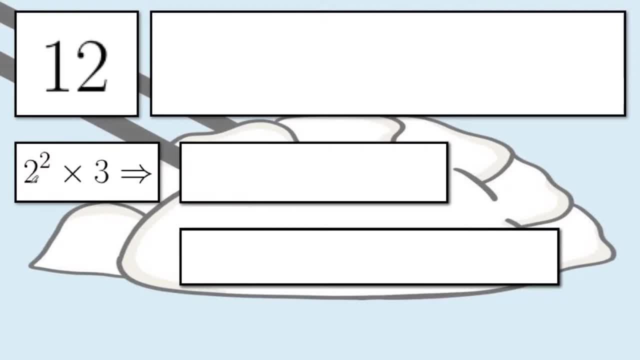 number in the prime factorization. So the power of 2 here is 2, and the power of 3 is actually 1.. So 3 raised to 1.. Now the next thing we have to do is we add 1 to all of the exponents. Now, since there 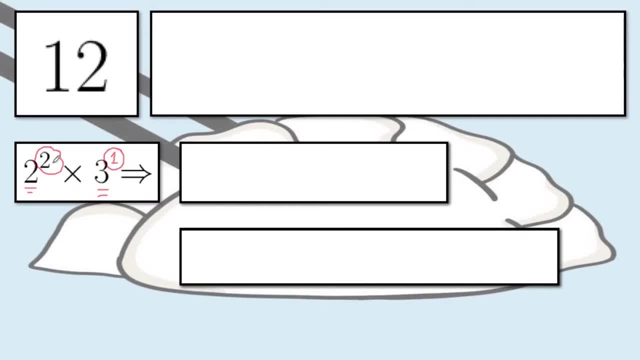 are two exponents, we will have two numbers that we multiply together, So it's not 2 and 1.. We add 1 to both of them, so it's going to become 2 plus 1 times 1 plus 1.. 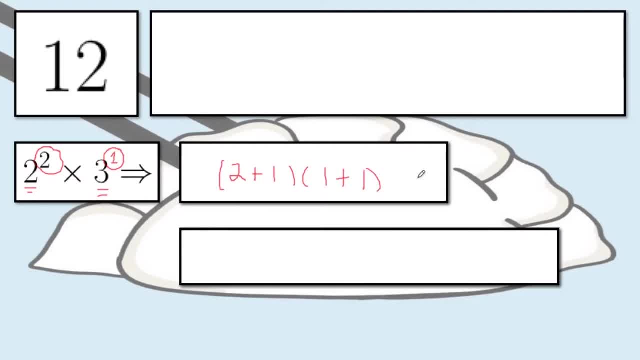 And this will give you the number of positive divisors. In fact, 2 plus 1 is 3, and 1 plus 1 is 2, so 3 times 2 would give us 6,, as shown a while ago when we listed down all of the. 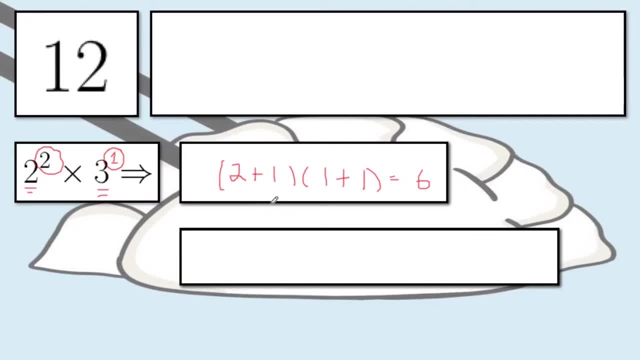 positive divisors of 12.. Now next for the sum of the positive divisors. Again, the number of factors is the same as the number of prime numbers that 12 is divisible by. so we expect 2 factors. Now to get the sum very simple, we start writing powers of primes from the lowest exponent. 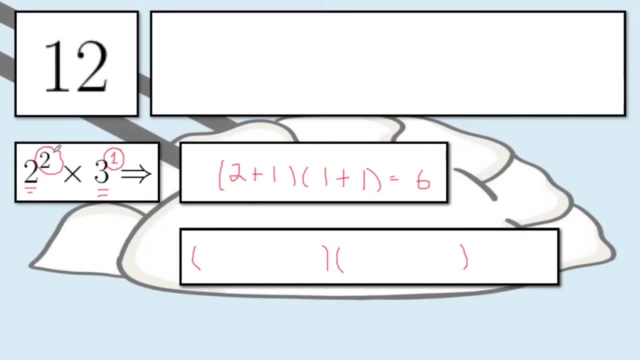 which is 0, to the highest exponent. So what do we mean by that? So let's take the example of the prime power of 2 here. So we start with 2 raised to 0,, which is also equal to 1, and then we write powers of 2 until we reach this term. 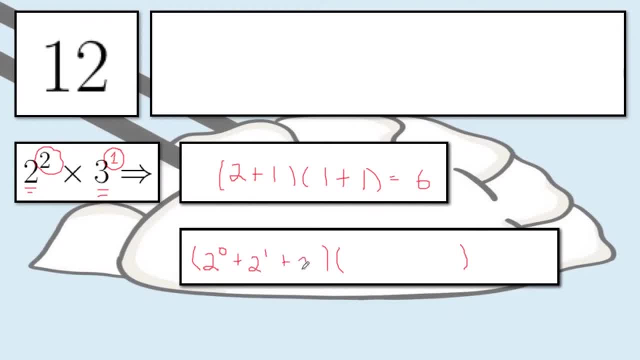 So 2 raised to 0, 2 raised to 1 and then 2 raised to 2.. And then we simply add them. Now suppose if this was a 2 raised to 3. instead, then we're going to add an additional 2 raised to 3,. 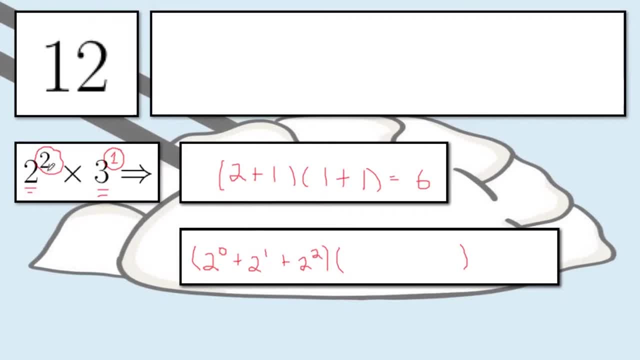 but since the power of the prime factor 2 here is 2, so we write from 2 raised to 0 up to 2 raised to 2.. Now for 3 raised to 1,. the lowest power of 3 is 3 raised to 0, and then the highest power is: 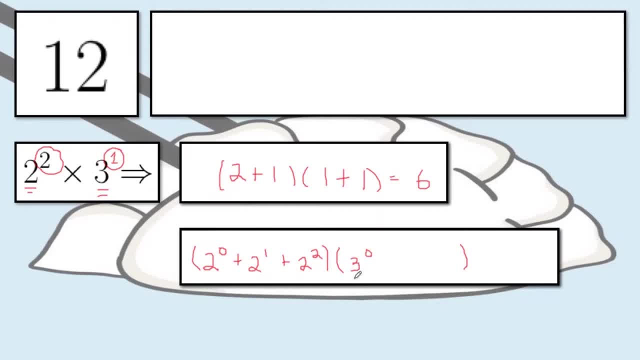 3 raised to 1, so we add powers of 3 from 3 raised to 3 raised to 1.. So it's just 3 raised to 0 plus 3 raised to 1.. Now 2 raised to 0 is: 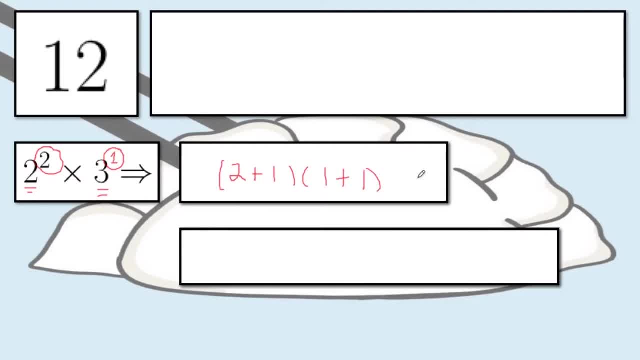 And this will give you the number of positive divisors. In fact, 2 plus 1 is 3, and 1 plus 1 is 2, so 3 times 2 would give us 6,, as shown a while ago when we listed down all of the. 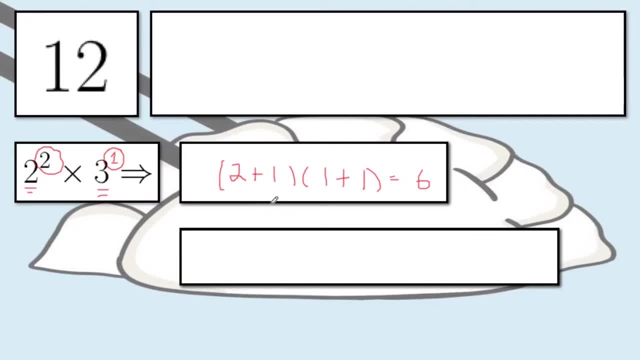 positive divisors of 12.. Now next for the sum of the positive divisors. Again, the number of factors is the same as the number of prime numbers that 12 is divisible by. so we expect 2 factors. Now to get the sum very simple, we start writing powers of primes from the lowest exponent. 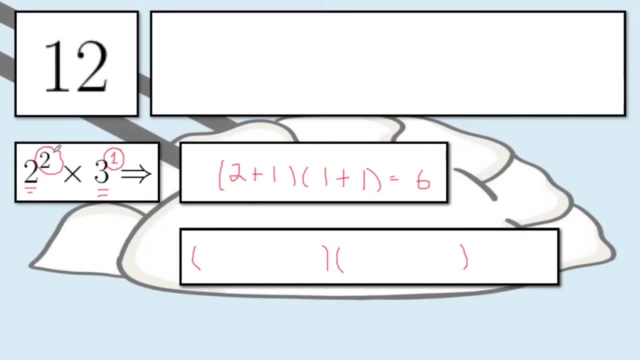 which is 0, to the highest exponent. So what do we mean by that? So let's take the example of the prime power of 2 here. So we start with 2 raised to 0,, which is also equal to 1, and then we write powers of 2 until we reach this term. 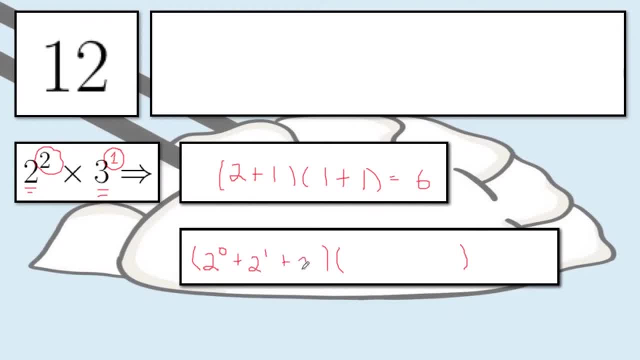 So 2 raised to 0,, 2 raised to 1, and then 2 raised to 2.. And then we simply add them. Now suppose if this was 2 raised to 3 instead, then we're going to add an additional 2 raised to 3,. 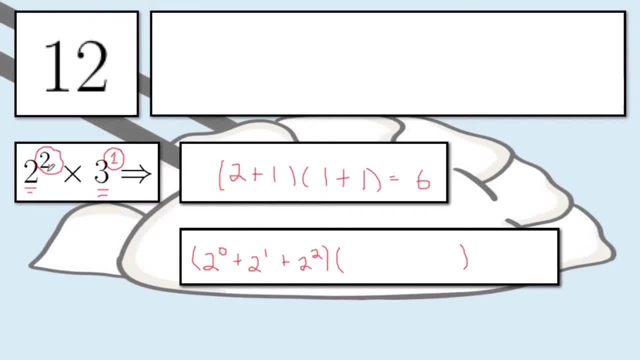 but since the power of the prime factor 2 here is 2, so we write from 2 raised to 0 up to 2 raised to 2.. Now for the 3 raised to 1, the lowest power of 3 is 3 raised to. 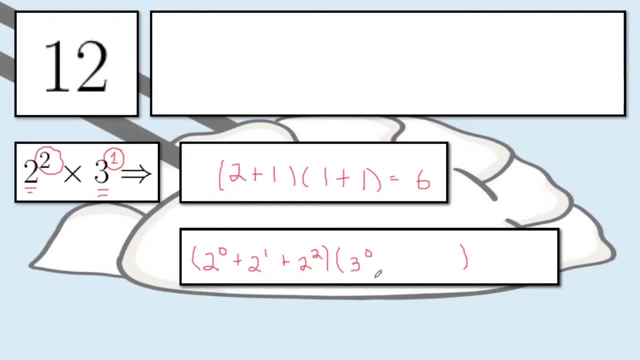 0, and then the highest power is 3 raised to 1, so we add powers of 3, from 3 raised to 1 up to 3 raised to 1.. So it's just 3 raised to 0 plus 3 raised to 1.. Now 2 raised to. 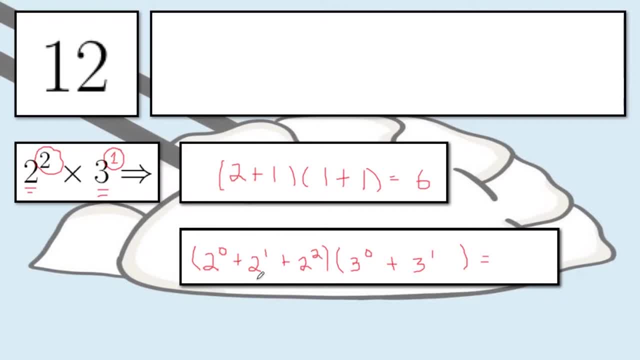 0 is 1,, 2 raised to 1 is 2, and 2 raised to 2 is 4,. so this will give us 7.. And 3 raised to 0 plus 3 raised to 1, that gives us 4.. And multiplying 7 and 4, we're going to get. 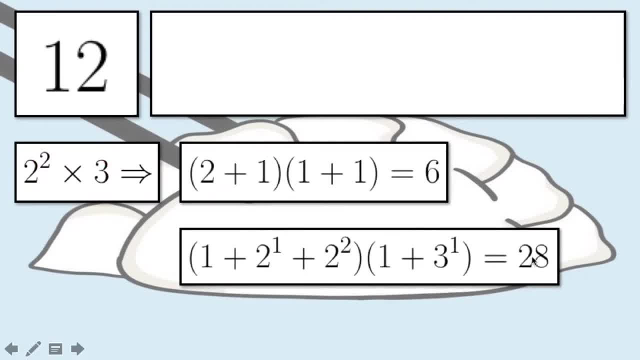 28, which are the two answers that we got. So, for the case of the positive integer, 12,, 6 is the number of positive divisors. let's say n is the number and 28 here is the sum of the positive divisors. Let's try to go to the next item. Alright, let's try to consider. 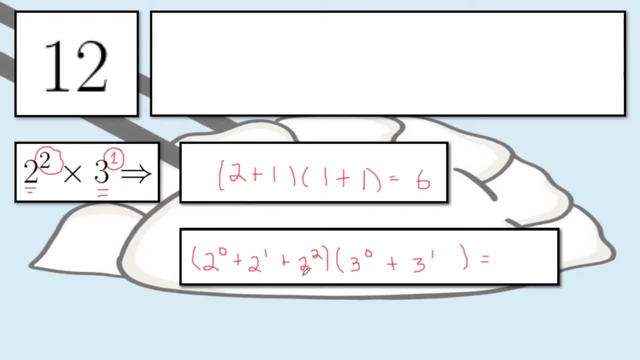 1, 2 raised to 1 is 2, and 2 raised to 2 is 4.. This will give us 7.. And 3 raised to 0 plus 3 raised to 1, that gives us 4.. And multiplying 7 and 4, we're going to get 28,, which are: 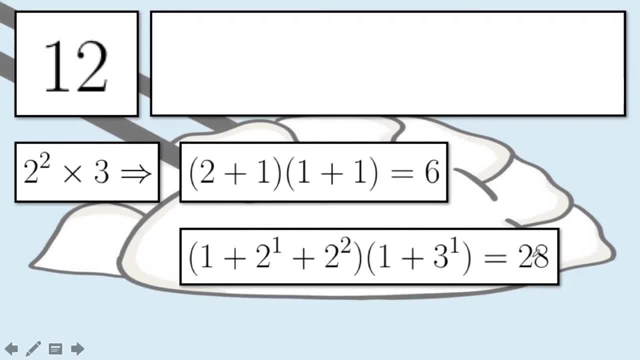 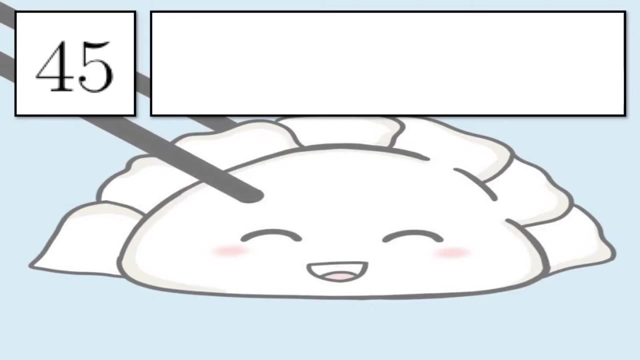 the two answers that we got. So, for the case of the positive integer, 12,, 6 is the number of positive divisors, that's, the n is the number, and 28 here is the sum of the positive divisors. Let's try to go to the next item. Alright, let's try to consider 45.. Now pause. 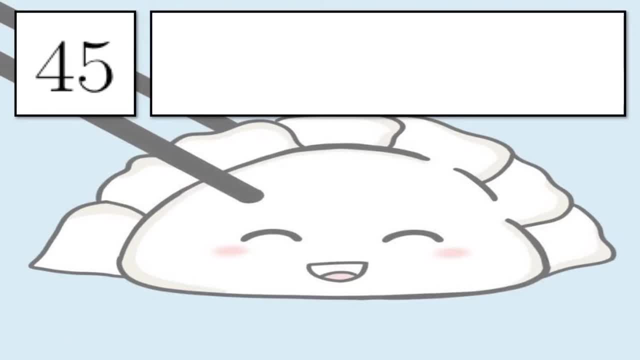 this video if you need some time to get the prime factorization or to list down all the positive divisors of 45. But if you're done, continue watching. Let's try to list down all the positive integer divisors of 45.. Well, 45 is divisible by 1,, 45 is divisible by 3,, 5,, 9,, 15, and. 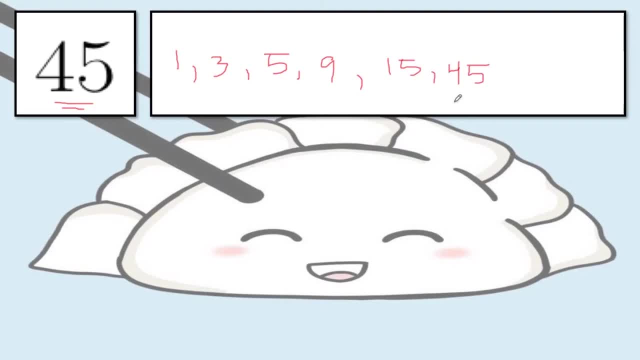 then 45. And you can verify that. there are no other numbers that 45 is divisible by. So if you want to get the number of positive divisors, that's going to be 6.. If you're going to get the sum, you simply add 1 plus 3 plus 5 plus 9 plus 15 plus 45, and this 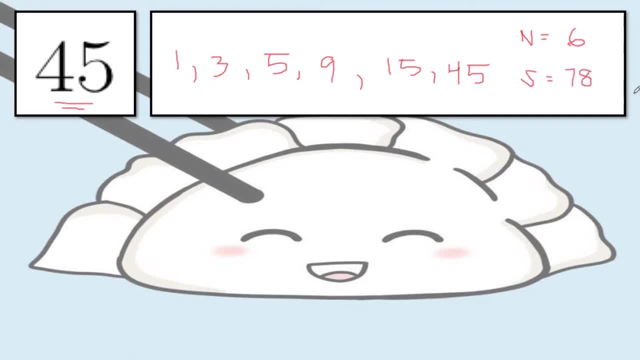 should give you an answer of 78.. Alright, now let's try to use the prime factorization method to verify whether or not 6 and 78 is correct. So we first get the prime factorization of 45. And then we're going to get the number of positive divisors that's going to be. 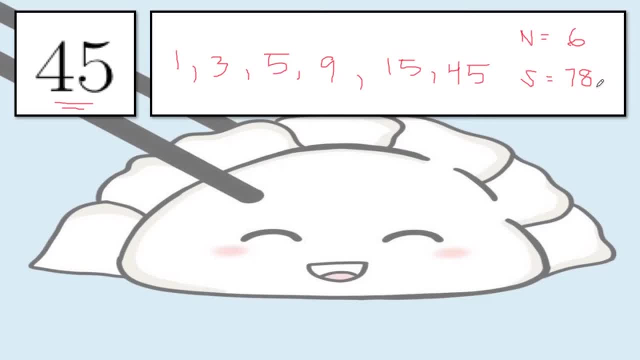 45. Now we know that 45 is 9 times 5, so 9 is 3 squared and we have a 5, so the prime factorization of 45 is 3 squared times 5.. Now let's deal with the number of positive. 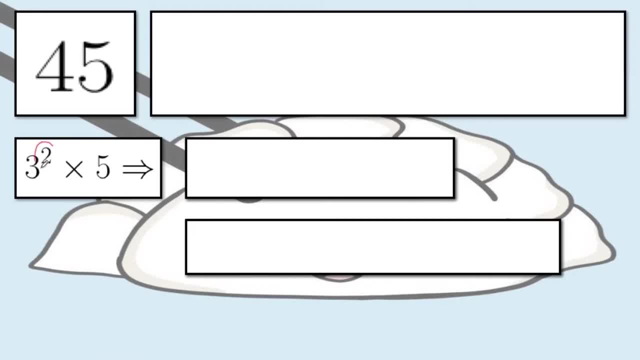 integer divisors. So same thing. we take the exponents now. the 5 here is an exponent of 1, so 2 and 1 are the exponents. so there are only two prime numbers. that 45 is divisible by. so we expect a product of two numbers here, So 2 and 1, so we want to add 1 to 2. 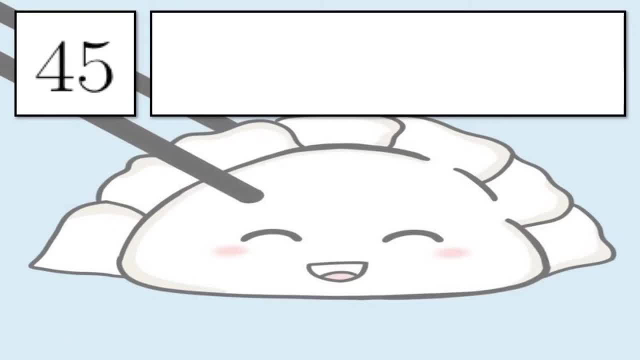 45. Now pause this video if you need some time to get the prime factorization or to list down all the positive divisors of 45. But if you're done, continue watching. Let's try to list down all the positive integer divisors of 45.. Well, 45 is divisible by 1,. 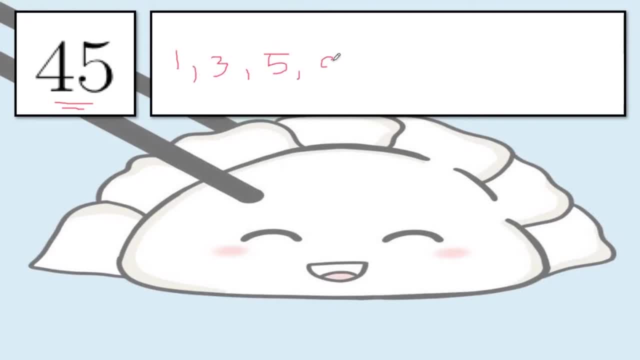 45 is divisible by 3,, 5,, 9,, 15, and then 45. And you can verify that there are no other numbers that 45 is divisible by. So if you want to get the number of positive divisors, 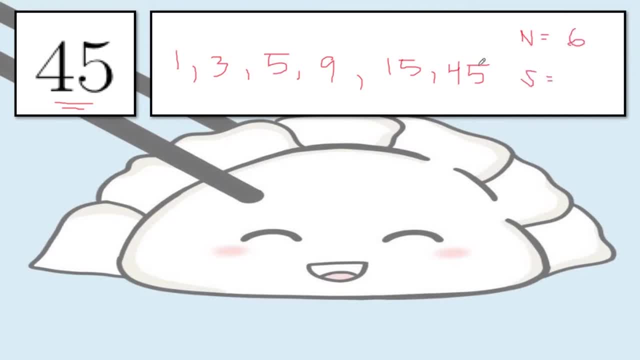 that's going to be 6.. If you're going to get the sum, that's going to be 8.. And if you're, we simply add 1 plus 3 plus 5 plus 9 plus 15 plus 45, and this should give you an answer of 78.. 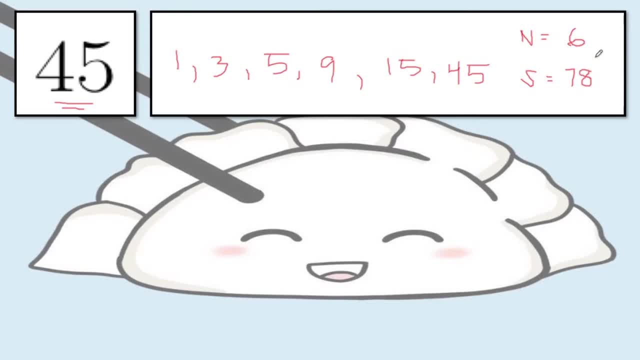 Alright, now let's try to use the prime factorization method to verify whether or not 6 and 78 is correct. So we first get the prime factorization of 45. Now we know that 45 is 9 times 5,. 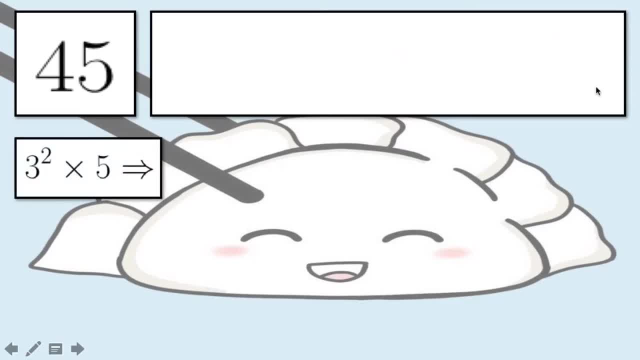 so 9 is 3 squared, and then we have a 5,. so the prime factorization of 45 is 3 squared times 5.. Now let's deal with the number of positive integer divisors. So same thing. we take the exponents. 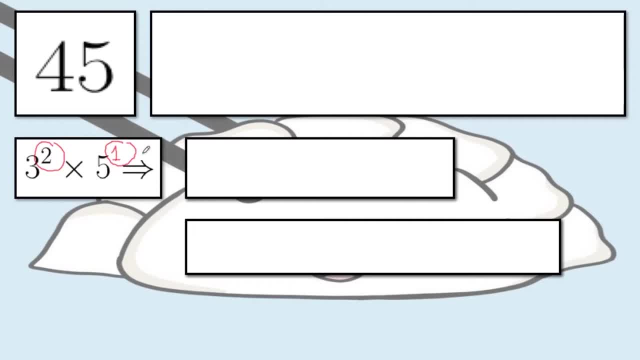 Now the 5 here is an exponent of 1, so 2 and 1 are the exponents. so there are only two prime numbers. that 45 is divisible by, so we expect a product of two numbers here, So 2 and 1.. 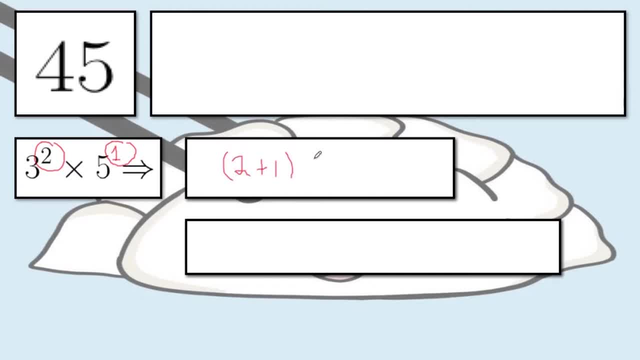 So we want to add 1 to 2 and 1, and then we multiply them. So this is the same case as the last example. So 2 plus 1 times 1 plus 1, that gives us 3 times 2, so it's 6.. 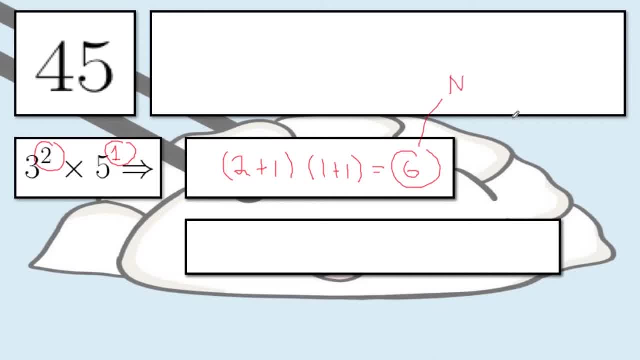 So the value of n that we got is actually correct. So this is the value of n. Now let's check whether or not the sum of the factors is actually 78.. Now, since we have powers of 3 and powers of 5,, 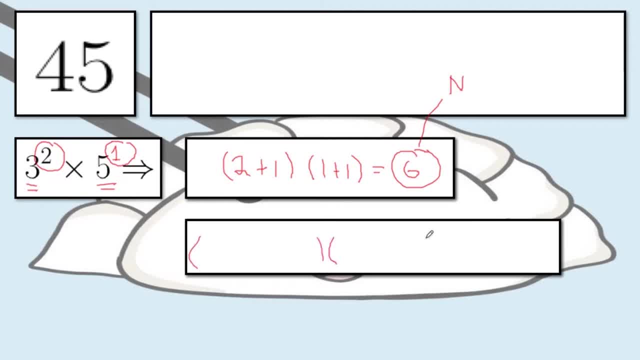 two prime numbers, so we expect a product of two numbers as well. Now for the power of 3,. we start with the lowest power, 3, raised to 0, and then we write until the largest power of 3,, which is 3 squared. 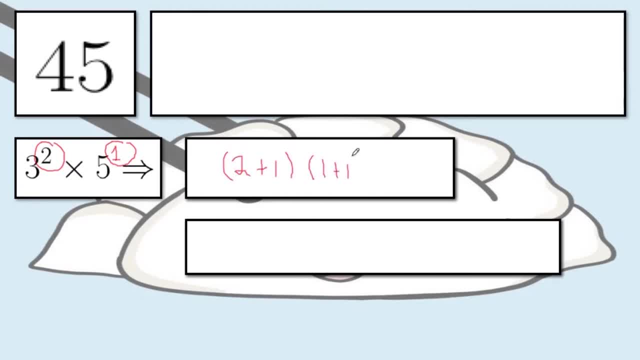 and 1, and then we multiply them. So this is the same case as the last example. so 2 plus 1 times 1 plus 1, that gives us 3 times 2, so it's 6.. So the value of n that we got. 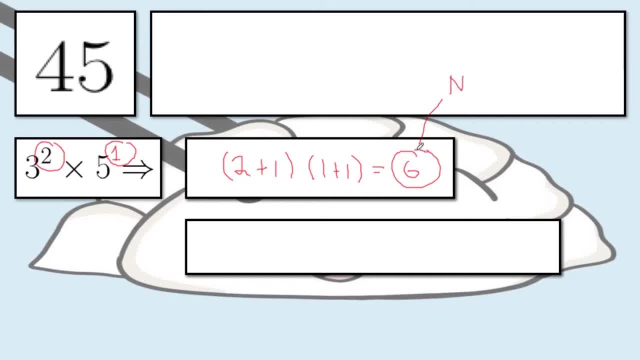 is actually correct. so this is the value of n. Now let's check whether or not the sum of the factors is actually 78.. Now, since we have powers of 3 and powers of 5, we're just going to have two prime numbers, so we expect a product of two numbers as well. Now, 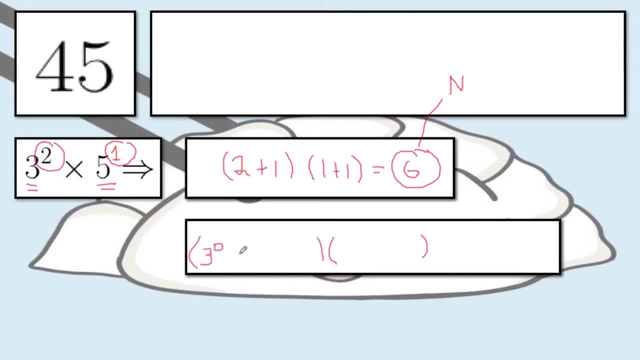 for the power of 3, we start with the lowest power, 3, raised to 0, and then we write until the largest power of 3, which is 3 squared. so we'll write until 3 squared. Now for 5. 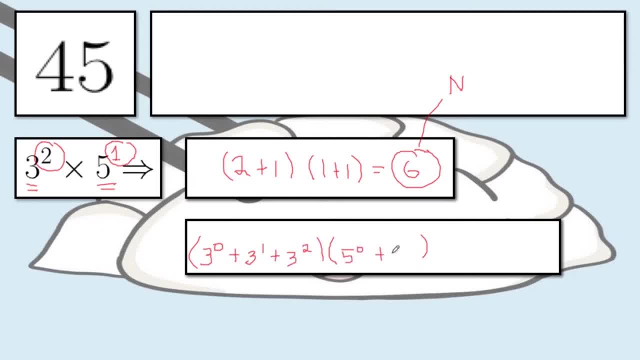 we start from 5 raised to 0 and we end at 5 raised to 1, so it's just 5 raised to 0 plus 5 raised to 1.. Now, 3 raised to 0 plus 3 raised to 1 plus 3 raised to 2, that's equal. 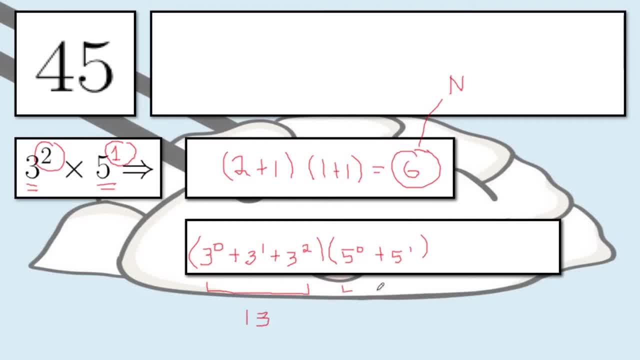 to 13.. 5 raised to 0 plus 5 raised to 1, that's equal to 6.. So 13 times 6,- you guessed it- it's 78. So we have 78 to be the sum of the divisors of 45, which is correct. 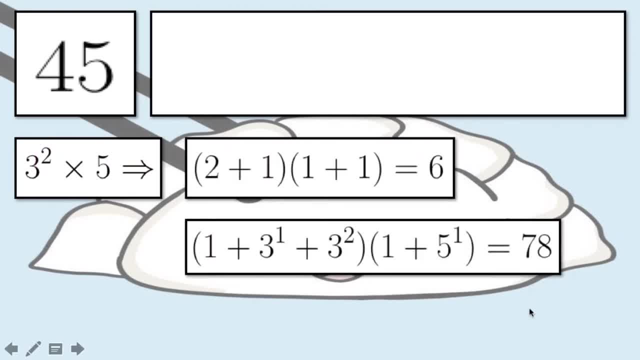 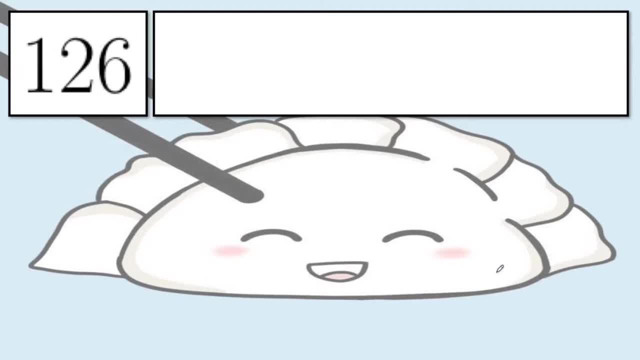 Let's try the next example. Let's try to deal with the number 126.. All right, we can still try to list them down. So 1,, 2,, 3,, 4 doesn't work. 6 works, 7 works. 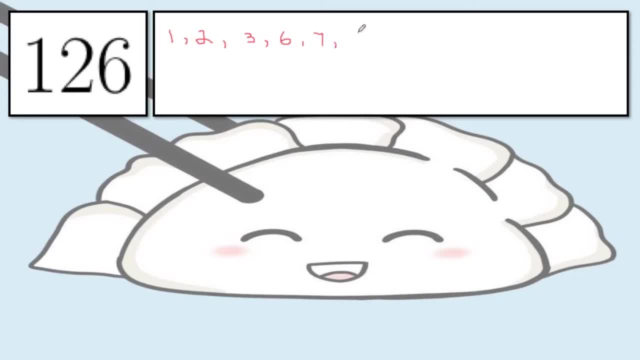 8 doesn't work. oh, 9 works. 10,, 11,, 12,, 14.. Okay, What else? 18,, 21,, 42,, 63, and then 126.. All right, take note as the numbers increase. obviously, chances are it's going to have more. 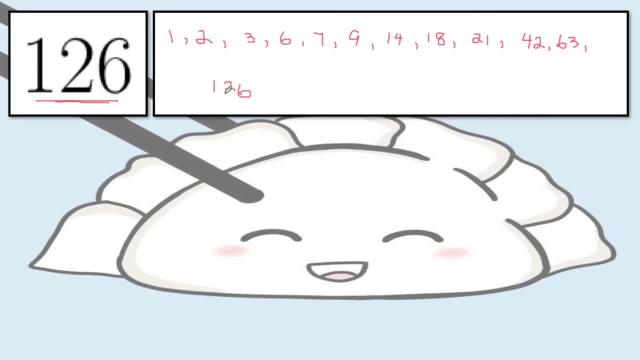 factors And I might have missed some of the numbers here, And that is the reason why most of the numbers in this example are not the same. Most of the numbers in this example are not the same. Most of the numbers in this example are not the same. 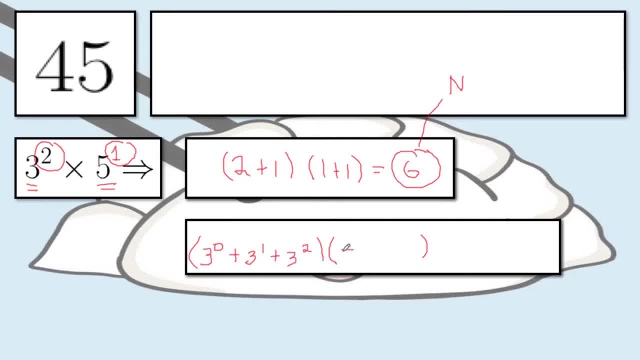 So we write until 3 squared Now for 5, we start from 5 raised to 0, and we end at 5 raised to 1, so it's just 5 raised to 0 plus 5 raised to 1.. 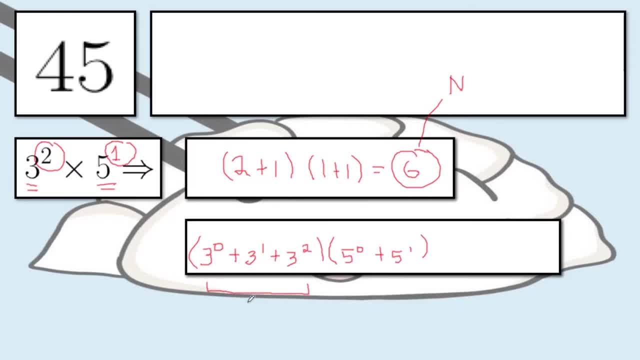 Now 3 raised to 0 plus 3 raised to 1 plus 3 raised to 2, that's equal to 13,. and then 5 raised to 0 plus 5 raised to 1, that's equal to 6.. 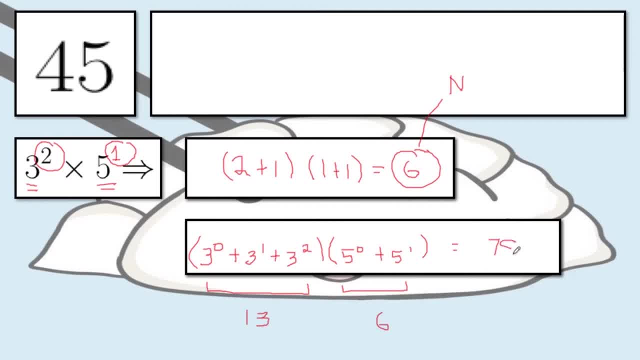 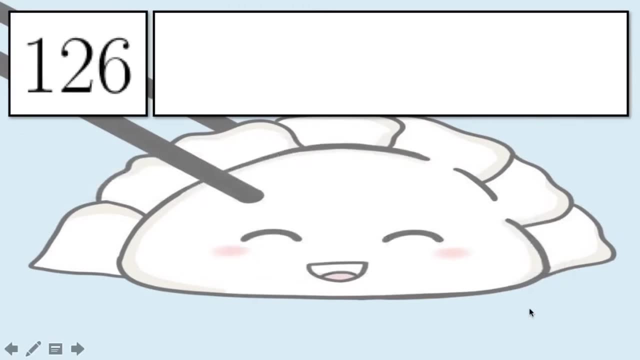 So 13 times 6, you guessed it, it's 78.. So we have 78 to be the sum of the divisors of 45, which is correct. Let's try the next example. Let's try to deal with the number 126. 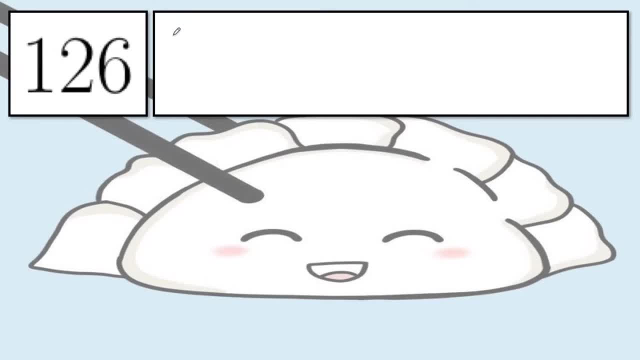 All right, we can still try to list them down. So 1,, 2.. 1,, 2,, 3,, 4 doesn't work. 6 works, 7 works, 8 doesn't work, oh, 9 works. 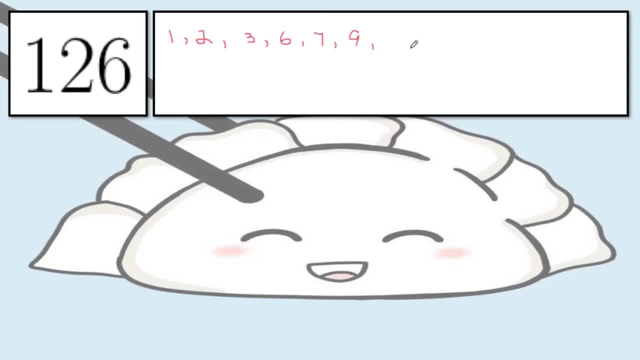 10,, 11,, 12,, 14,- what else? 18, 21.. 42,, 63, and then 126.. All right, take note as the numbers increase, obviously chances are it's going to have more factors. 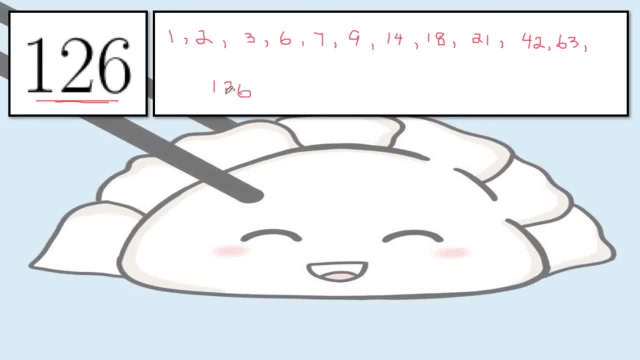 and I might have missed some of the numbers here, and that is the reason why learning this shortcut or trick is very essential, because when dealing with larger numbers, it will be almost impossible for you to count the number of positive integer divisors, let alone just 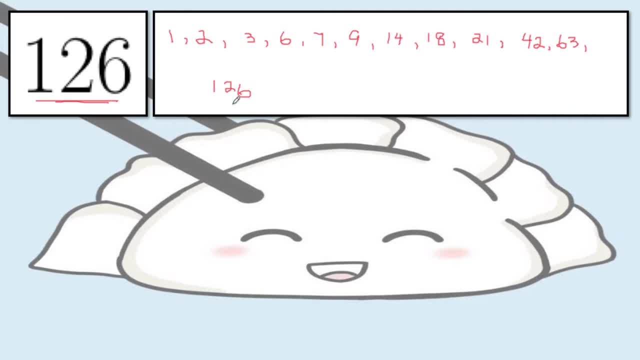 Let's add all of them. all right, So let's just try to get the value of n. So I have 1,, 2,, 3,, 4,, 5,, 6,, 7,, 8,, 9,, 10,, 11,, 12.. 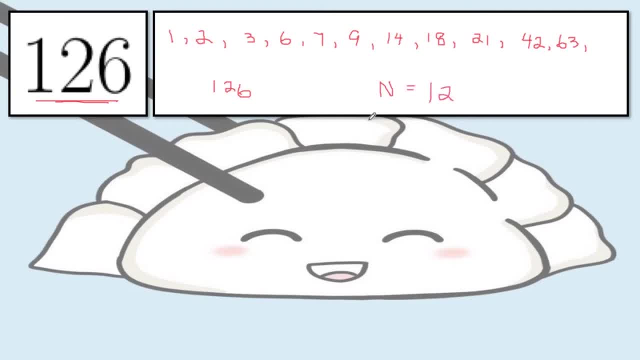 So from counting I get that n equals 12.. So let's just verify if it's correct. So same thing. we must get the prime factorization, So 126,. okay, I see that the sum of the digits is 9,. 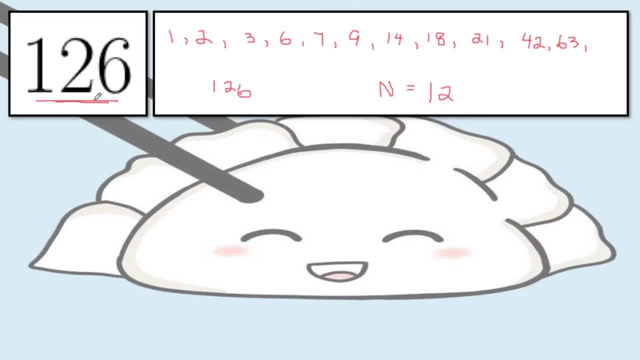 so I know the number is divisible by 9.. So it's going to involve some 3-squared prime factorization. So okay, we have this. That's the prime factorization. So 2 times 3-squared times 7.. 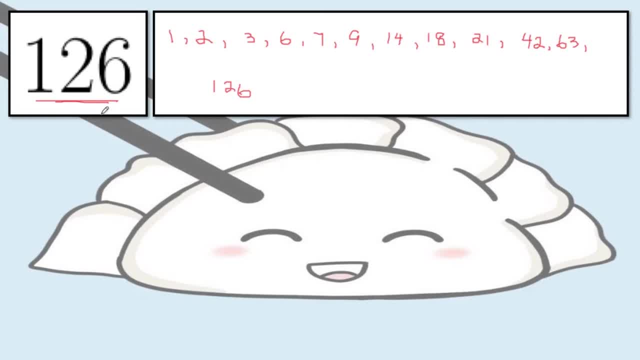 Most of the numbers in this example are not the same. Learning this shortcut or trick is very essential because when dealing with larger numbers, it will be almost impossible for you to count the number of positive integer divisors, let alone just add all of them. 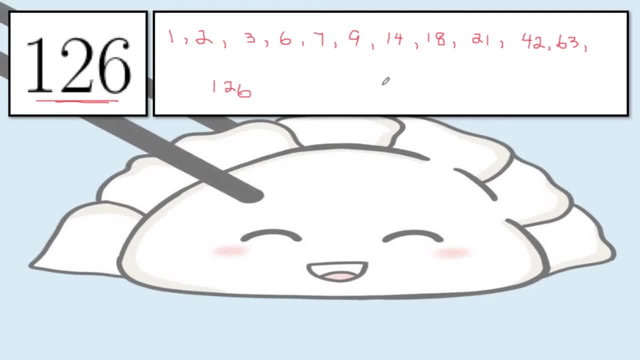 All right, So let's just try to get the value of n. So I have 1,, 2,, 3,, 4,, 5,, 6,, 7,, 8,, 9,, 10,, 11,, 12.. 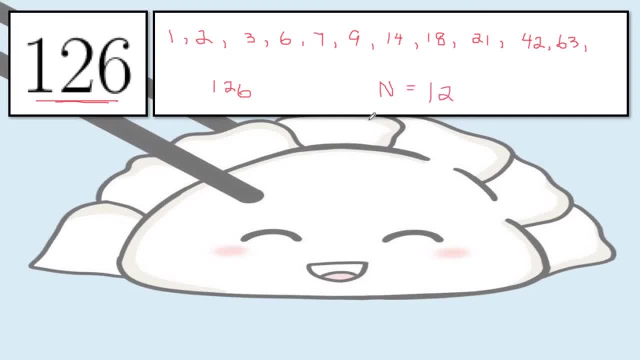 So from counting I get that n equals 12.. So let's just verify if it's correct. So same thing. we must get the prime factorization, So 126,. okay, I see that the sum of the digits is 9.. 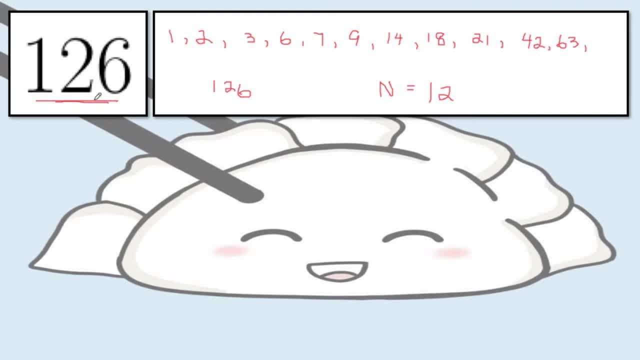 So I know the number is divisible by 9.. So it's going to involve some 3 squared prime factorization. So, okay, we have this as the prime factorization, So 2 times 3 squared times 7.. So now we have 3 prime factors. 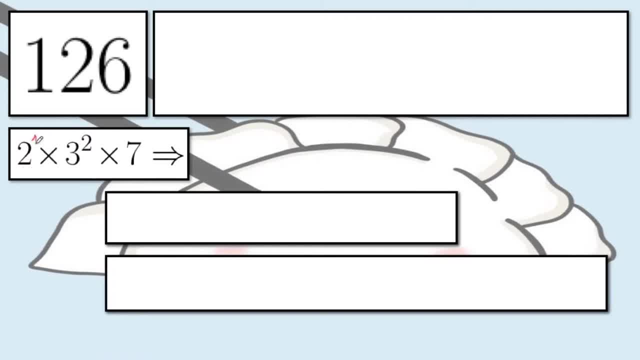 So let's take the exponents. So that's 2 raised to 1,, 3 raised to 2, and 7 raised to 1.. Now we need to check The number of positive integer divisors. We add 1 to the exponent. 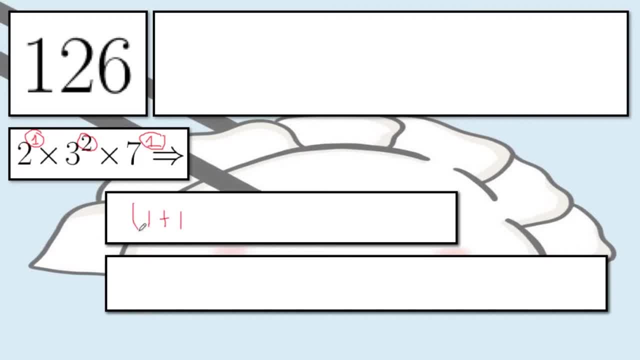 So 1 plus 1.. Now, since there are 3 exponents, it's a product of 3 different numbers. So 1 plus 1 times 2 plus 1 times 1 plus 1.. And this gives us 2 times 3 times 2.. 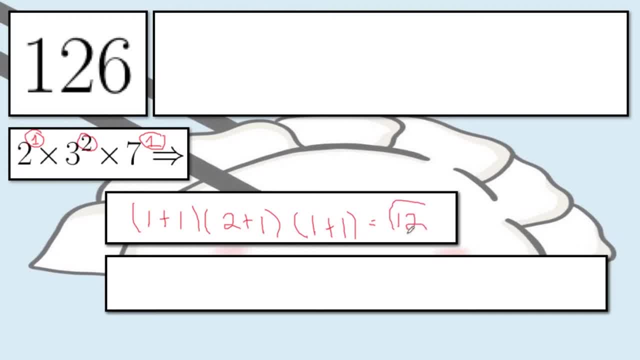 And this gives- oh, this gives us 12.. So the value of n that we got from counting was actually correct, But as seen by the number of positive integer divisors, it's very tedious for us to add all 12.. So let us apply this method instead. 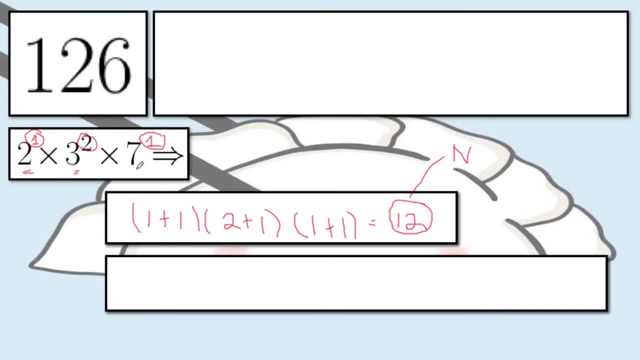 So, starting with the power of 2, again, since there are 3 prime factors, sorry, there are 3 prime numbers- that 1, 26 is divisible by, we expect a product of 3 terms Right for 2 raised to 1,. we start from the smallest factor, sorry, the smallest power. 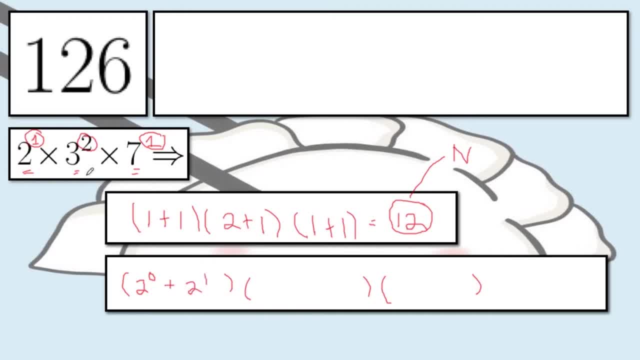 of 2.. So 2 raised to 0 plus 2 raised to 1.. So for 3 squared, we start from 3 raised to 0.. And then 3 raised to 1.. And then 3 raised to 2.. 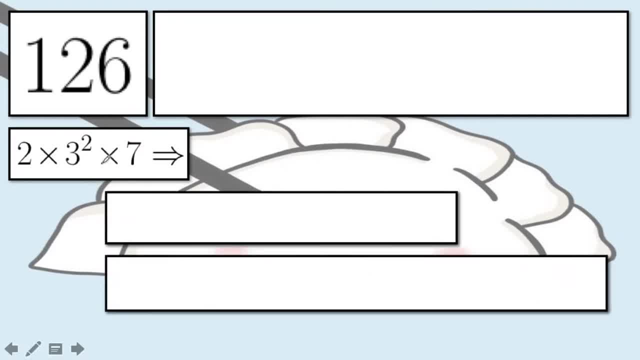 So now we have 3 prime factors. So let's take the exponents and that's 2 raised to 1,, 3 raised to 2, and 7 raised to 1.. Now we need to check the number of positive integer divisors. 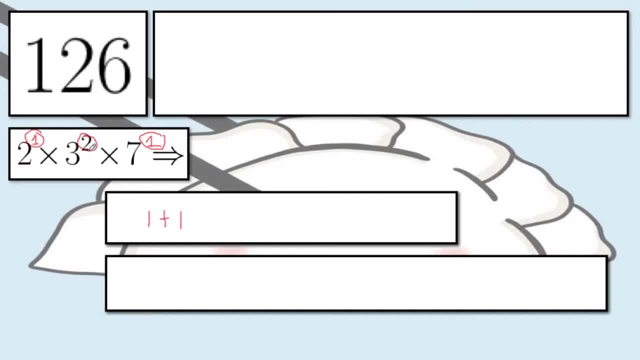 We add 1 to the exponent, so 1 plus 1.. Now, since there are 3 exponents, it's a product of 3 different numbers, So 1 plus 1, times 2 plus 1, times 1 plus 1.. 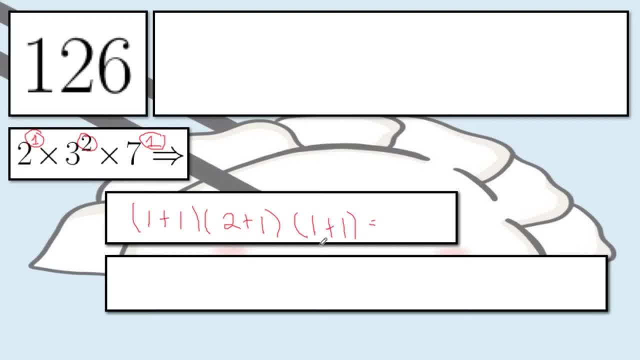 And this gives us 2 times 3 times 2.. And this gives- oh, this gives us 12.. So the value of n that we got from counting was actually correct, But as seen by the number of positive integer divisors, 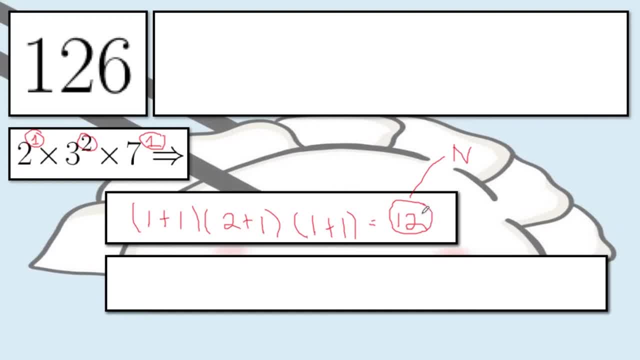 it's very tedious for us to add all 12. So let us apply this method instead. So, starting with the power of 2, again, since there are 3 prime factors- sorry, there are 3 prime numbers- that 126 is divisible by. 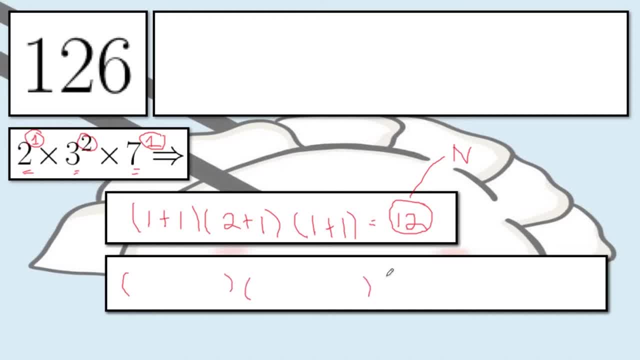 we expect a product of 3 terms, Right for 2 raised to 1, we start from the smallest factor, sorry, the smallest power of 2.. So 2 raised to 0 plus 2 raised to 1.. 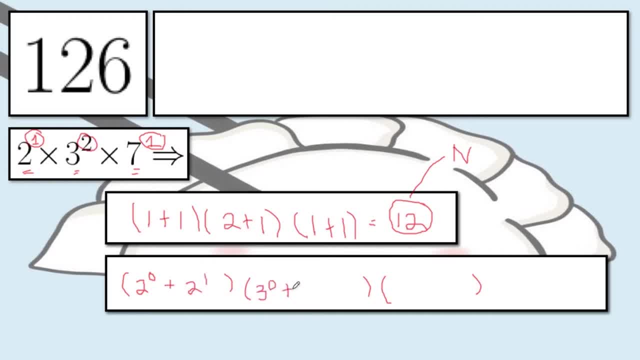 So for 3-squared, we start from 3 raised to 0, and then 3 raised to 1, and then 3 raised to 2.. For 7 raised to 1, it's 7 raised to 0, plus 7 raised to 1.. 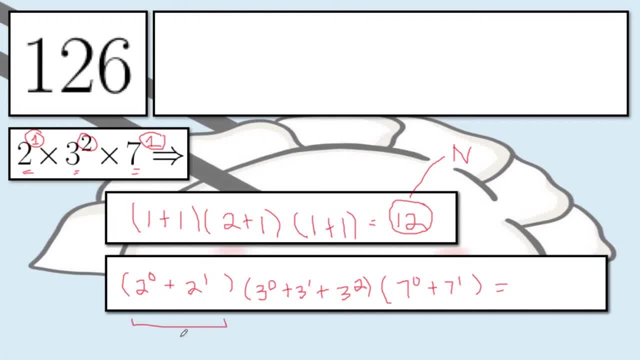 Now this will give us 3,, since 1 plus 2.. This will give us 13,, and this will give us 8.. So what we have to do is multiply 3 times 13 times 8, and this gives us 312. 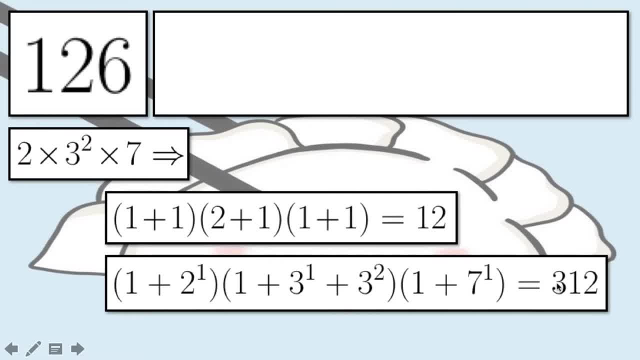 Now let's check if our answer is correct. Yes, it is. So note how, as the numbers increase, obviously the prime factorization is going to get more common. the prime factorization is going to get more complex, so the number of devices is going to increase, let alone the sums. 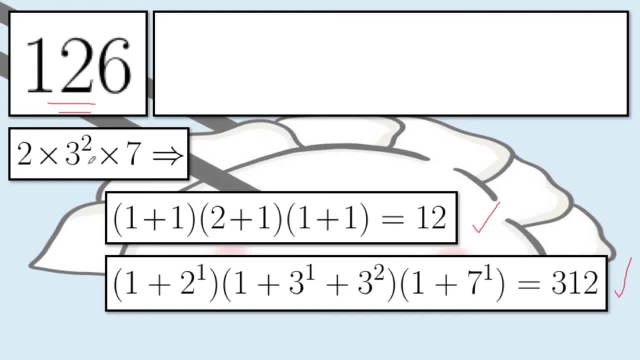 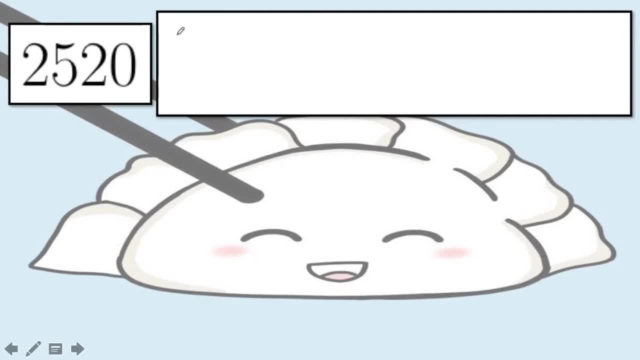 So what more? in the next example, when the number has become a 4-digit number, So 2520,, I don't think we want to write anything because after 1,, 2, there's just a lot of numbers to cover, from 1 to 2520. 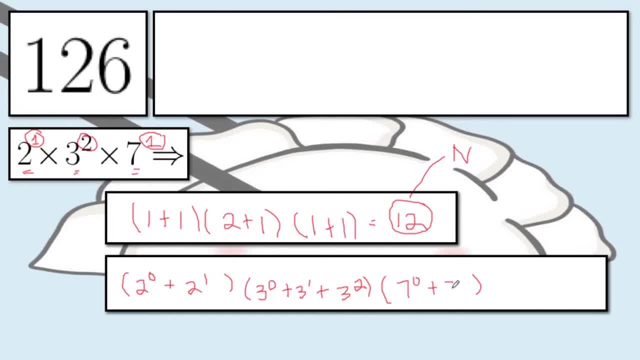 For 7 raised to 1, 7 raised to 0 plus 7 raised to 1.. Now this will give us 3, since 1 plus 2.. This will give us 13. And this will give us 8.. 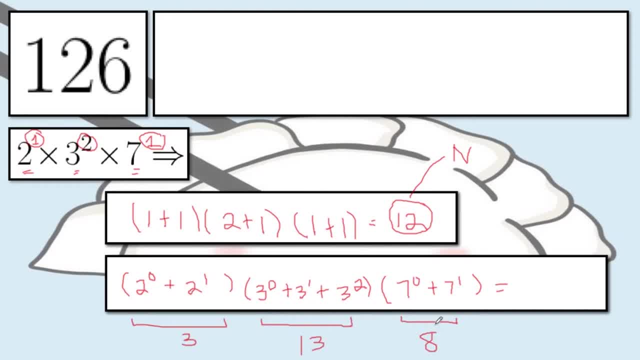 So what we have to do is multiply 3 times 13 times 8. And this gives us 312.. Now let's check If our answer is correct. yes, it is. So note how, as the numbers increase, obviously the prime factorization is going to get more. 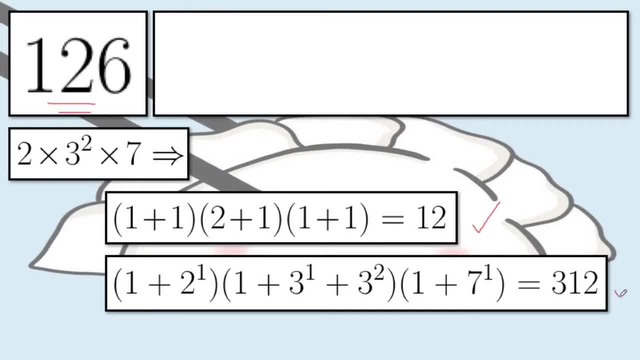 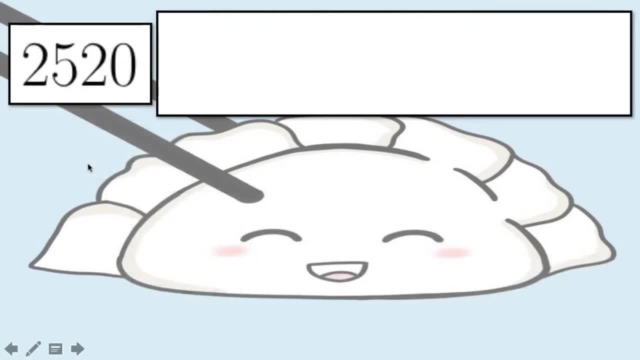 complex. So the number of devices is going to increase, let alone the sums. So what more in the next example, when the number has become a four-digit number? So 2,, 5,, 20, I don't think we want to write anything, because after 1,, 2, there's just. 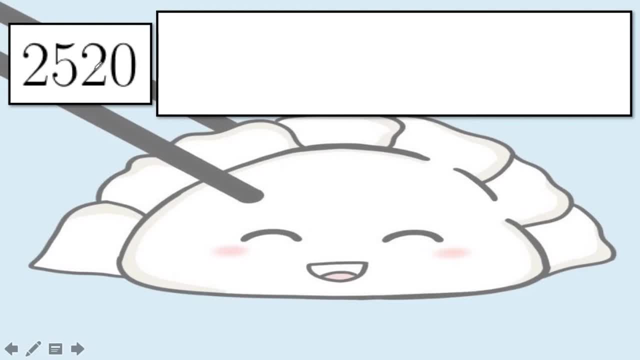 a lot of numbers to cover, So we want to cover from 1 to 2,520.. So let us just go directly into getting the prime factorization. Alright, you can pause this video and give yourself some time to prime factorize. 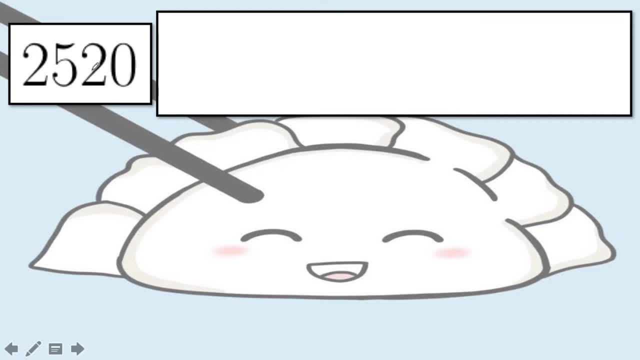 But if you're done, I'm going to show the prime factorization right now. So the prime factorization of 2,520 is 2 cubed times 3 squared times 5 times 7.. Note how there are four prime factors now. 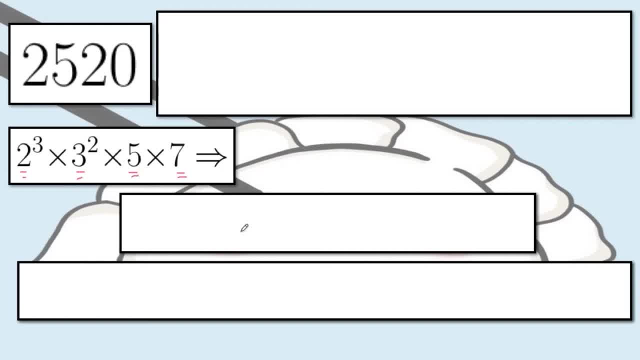 So it is expected that both expressions here will have a product of four numbers. So same thing. we take the exponents 3,, 2, 1, and then 1.. So we would expect our answer to become 3 plus 1 times 2 plus 1 times 1 plus 1 times. 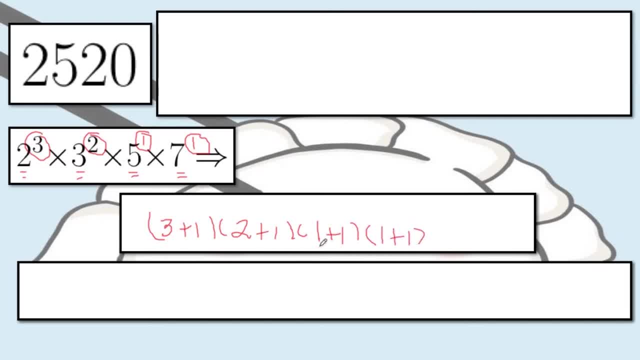 1 plus 1.. So it's equal to 4 times 3 times 2 times 2.. This gives us 48. So if we are to list down the positive integer divisors of 2,520, we'll have to list 48,, let alone add all of them. 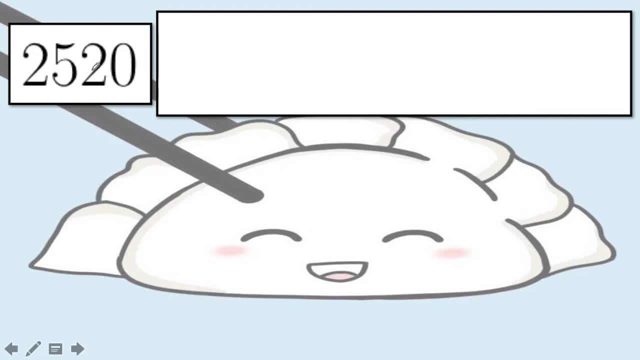 So let us just go directly into getting the prime factorization Right. you can pause this video and give yourself some time to prime factorize, but if you're done, I'm going to show the prime factorization right now. So the prime factorization of 2520 is 2 cubed times 3 squared times 5 times 7.. 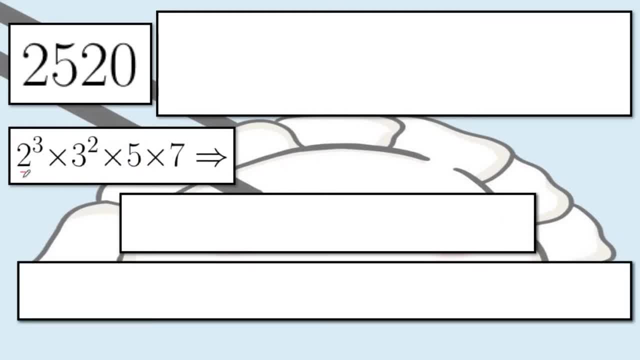 Note how there are 4 prime factors now. So it is expected that both expressions here will have a product of 4 numbers. So same thing. we take the exponents 3,, 2,, 1, and then 1.. 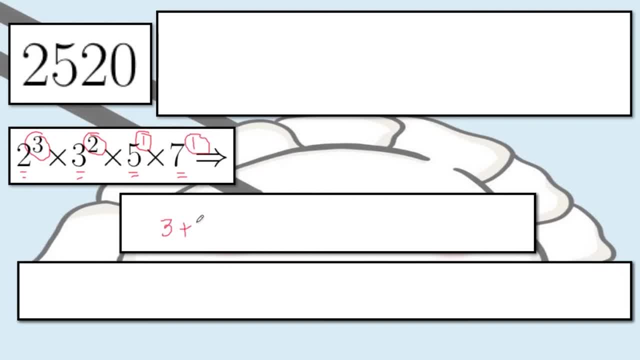 So we would expect our answer to become 3 plus 1 times 2 plus 1 times 1 plus 1 times 1 plus 1.. So it's equal to 4 times 3 times 2 times 2.. 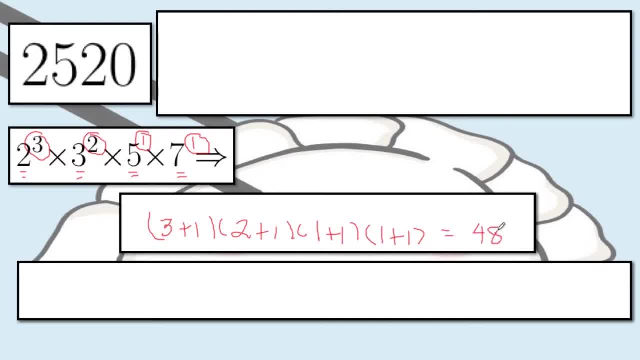 This gives us 48. So if we are to list down the positive integer divisors of 2520, we'll have to list 48, let alone add all of them and get the sum of them. So this method is indeed very helpful. 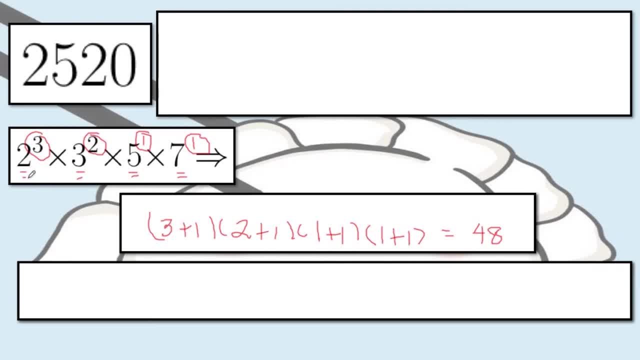 So next for the sum of the roots, sorry for the sum of the positive integer divisors. again, we expect 4 factors. Now for 2 cubed, we start from the lowest factor, 2, raised to 0,. 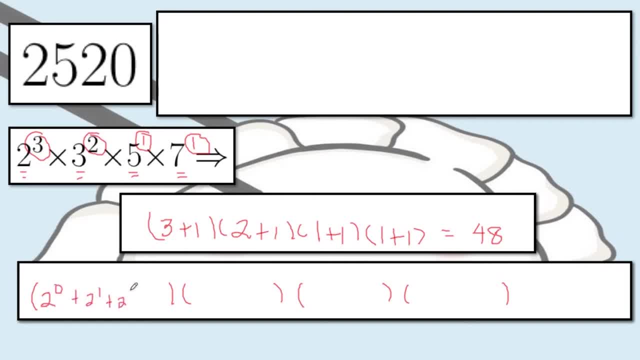 then we add 2 raised to 1, 2 raised to 2, 2 raised to 3.. For the 3 squared, we start from 3 raised to 0, plus 3 raised to 1, plus 3 squared. 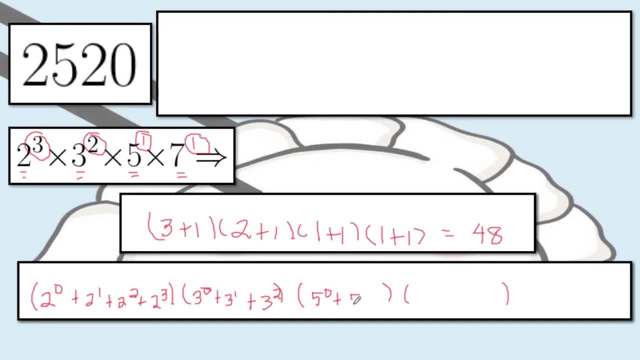 For 5 raised to 1,, 5 raised to 0, plus 5 raised to 1.. For 7,: 7 raised to 0, plus 7 raised to 1.. Now, this number is obviously very big. 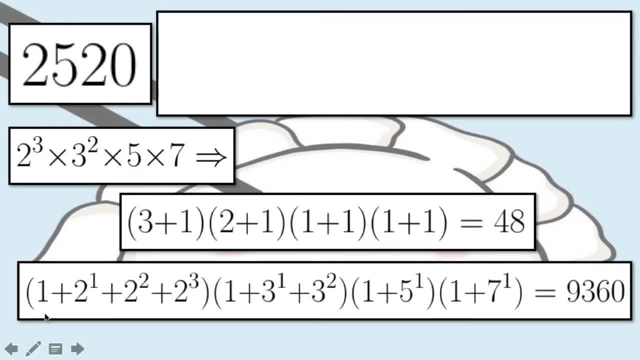 and in fact we have the answer here to be 9360.. So again, we have this 48 to be the number of the root, we have this 48 to be the number of positive integer divisors. the 9360 here would be the sum of the positive integer divisors. 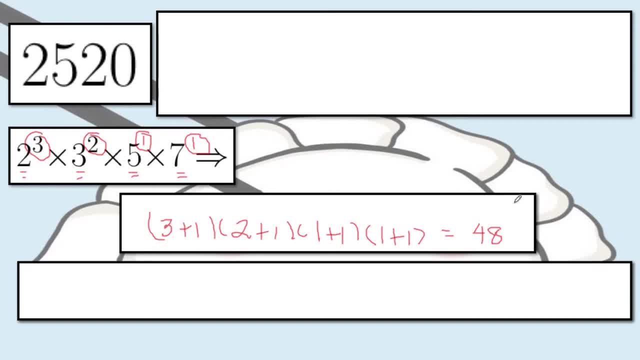 and get the sum of the divisors. So this method is indeed very helpful. So next for the sum of the positive integer divisors. again we expect four factors. Now for 2 cubed, we start from the lowest factor, 2, raised to 0.. 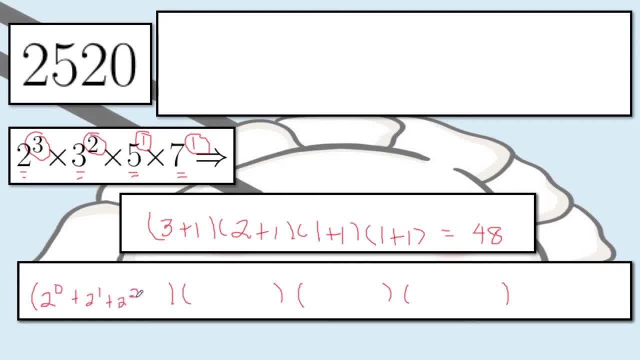 Then we add 2 raised to 1, 2 raised to 2, 2 raised to 3.. For the 3 squared, we start from 3 raised to 0, plus 3 raised to 1, plus 3 squared. 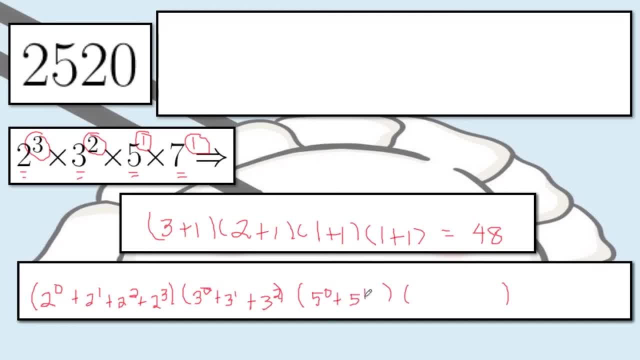 For 5 raised to 1,, we add 5 raised to 0, plus 5 raised to 1.. For 7,, 7 raised to 0, plus 7 raised to 1.. Now this number is obviously very big and in fact we have the answer here to be 99,000. 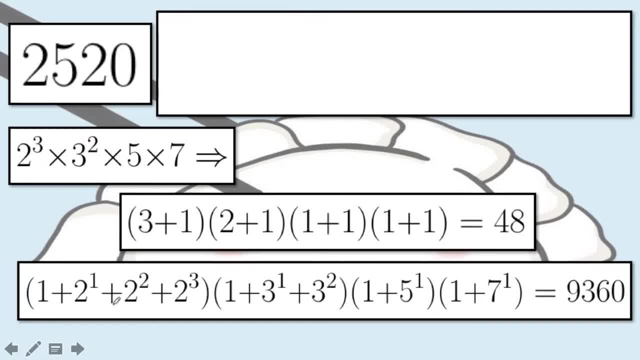 Yes, We did it. Yes, So again we have this 48 to be the number of positive integer divisors. the 9360 here would be the sum of the positive integer divisors. Alright, for the final practice item. let us try to get the number of factors and the 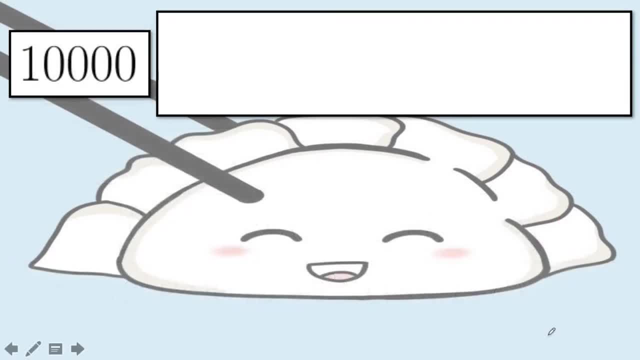 sum of the factors of 10,000.. So it's already a five-digit number, so we don't want to list down, I guess. So prime factorization of 10,000, that's actually very simple because it's just 10 raised to. 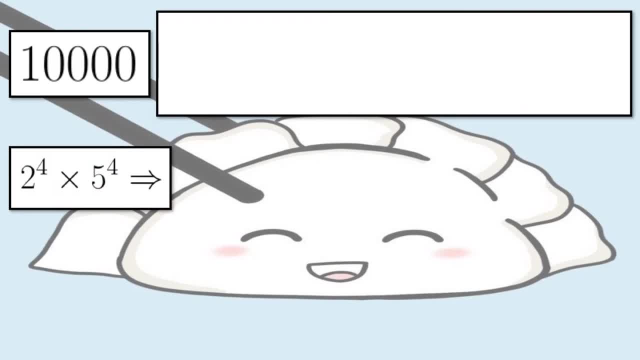 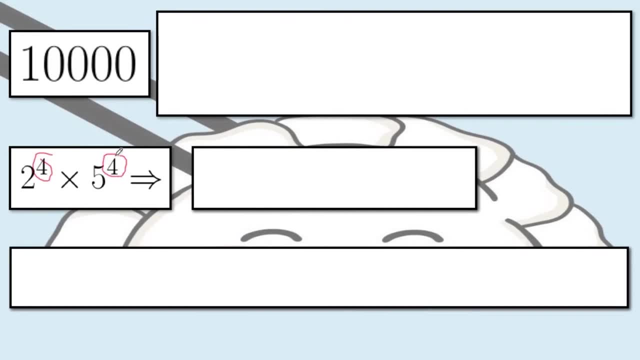 4, so we have 2 raised to 4 times 5 raised to 4.. Now we expect, since the exponents are 4 and 4, hopefully you guys are getting along quickly now- So 4 and 4, we expect this to become 4 plus 1 times 4 plus 1.. 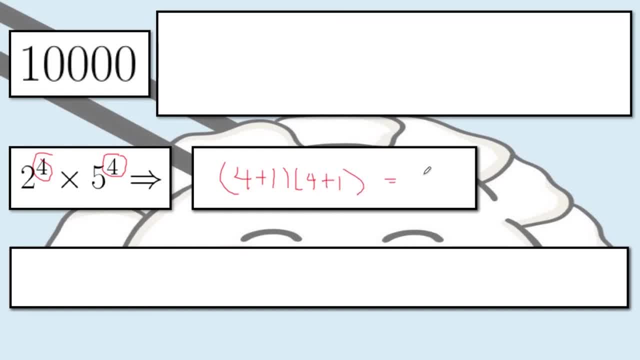 And this will give us 25, because it's just 5 times 5.. And for the bottom, we expect 2 raised to 0 plus 2 raised to 1, until 2 raised to 4 times 2 raised to 0, plus until 2 raised to 4, multiplied by 5 raised to 0 plus so on and so forth, until 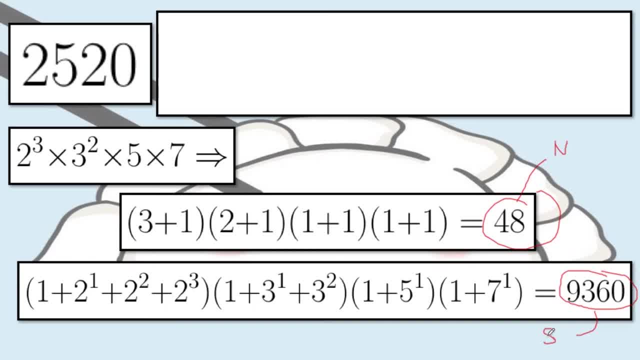 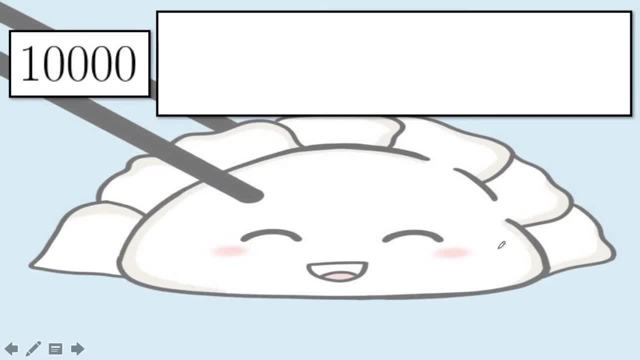 Alright, for the final practice item. let us try to get the number of factors and the sum of the factors of 10,000.. So it's already a 5-digit number. so well, we don't want to write any. 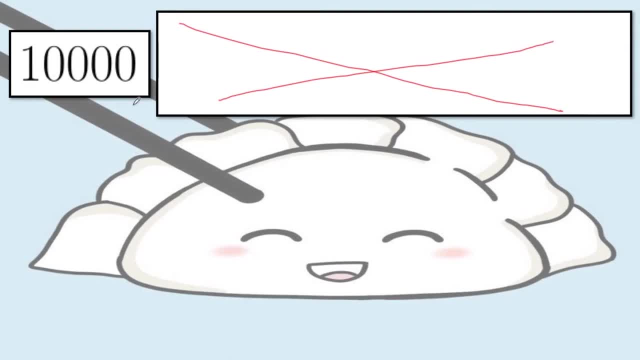 we don't want to list down, I guess. So prime factorization of 10,000, that's actually very simple because it's just 10 raised to 4.. We have 2 raised to 4, times 5 raised to 4.. 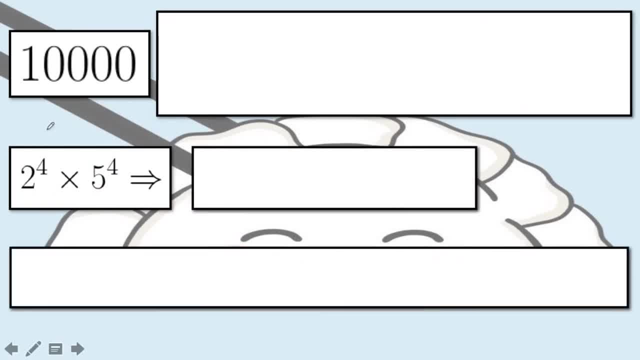 Now we expect, since the exponents are 4 and 4, hopefully you guys are getting along quickly now- So 4 and 4, we expect this to become 4 plus 1, times 4 plus 1, and this will give us 25,. 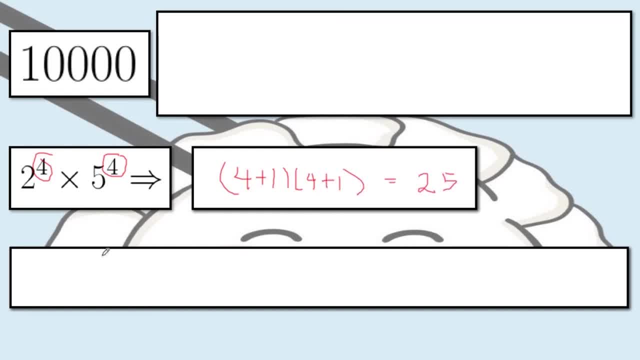 because it's just 5 times 5.. And for the bottom, we expect 2 raised to 0, plus 2 raised to 1, until 2 raised to 4, times 2 raised to 0, plus until 2 raised to 4,. 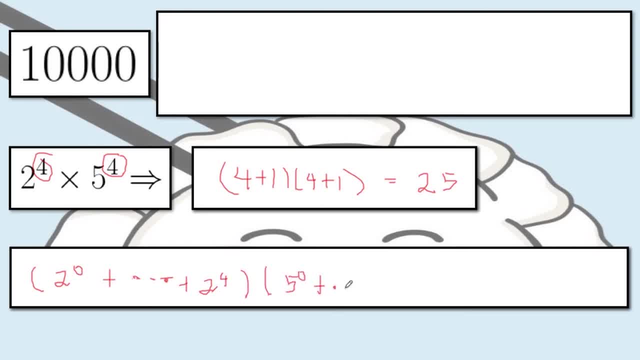 multiplied by 5, raised to 0,, plus so on and so forth, until 5 raised to 4.. And in fact we will be correct. So 4 plus 1, times 4 plus 1, and gives us 25.. 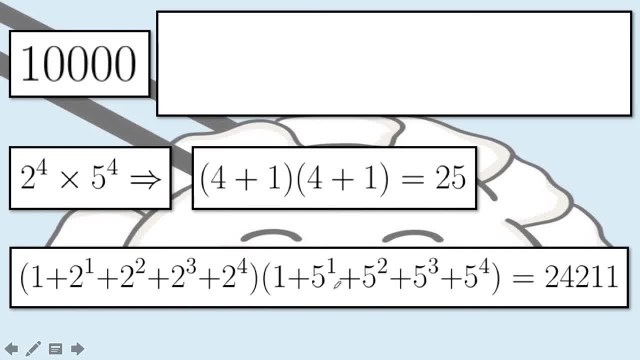 And here we have the sum of the roots, sorry, the sum of the positive integer divisors, So 25. here is the number of positive divisors of 10,000, and 24,211 over. here is the number is the sum of the positive integer divisors. 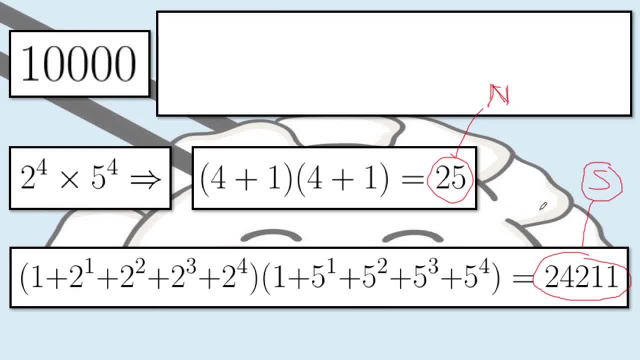 Alright, So hopefully you guys learned something from this video. Hopefully you'll be able to utilize the trick in getting the number of divisors or even the sum of the divisors quickly. Now, as a final item, you guys can solve and answer in the comment section down below. 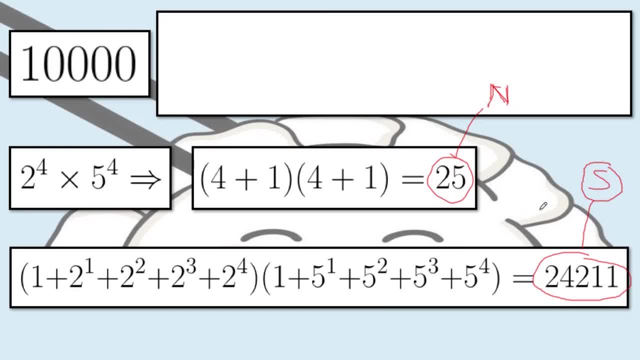 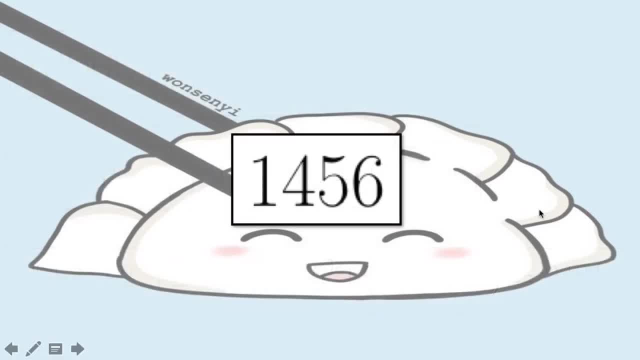 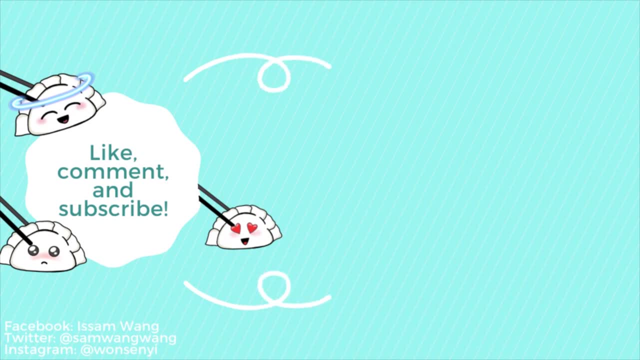 Try to get the number of positive integer divisors as well as the sum of the positive integer divisors of the number 1,456.. Alright, I'll see you again in the next video. Bye, bye. Thanks for watching.